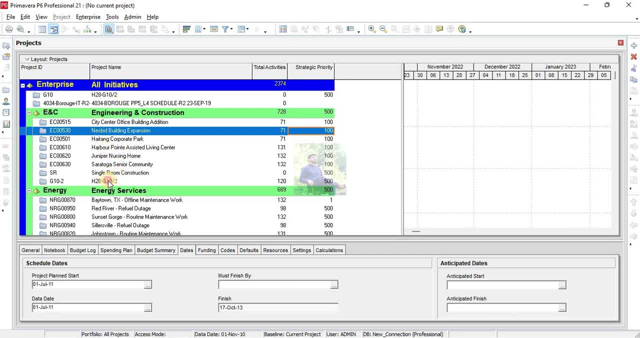 Primavera software. I will come to this window Now. I want to develop a schedule of 25 by 50 house, which will be ground floor plus first floor plus maamti. In ground floor there will be two rooms and on first floor there will be 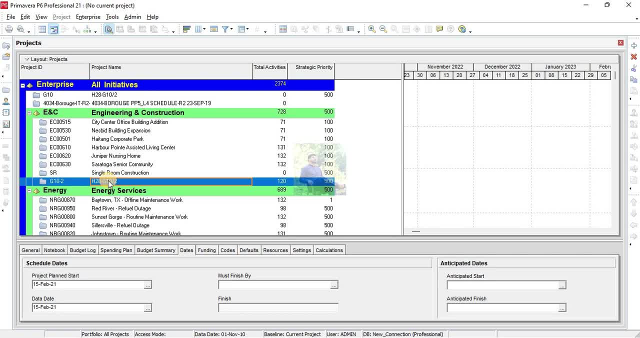 two rooms. On both ground floor and first floor there will be a dry room and a kitchen, and and on rooftop there will be a servant quarter which will include one room and a washroom, attached washroom and a small kitchen. so this will be layout of the house. now I want to 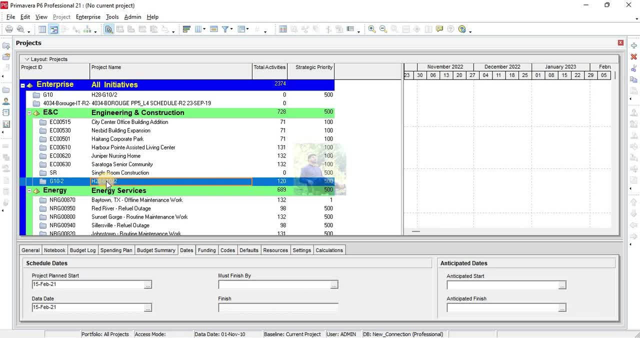 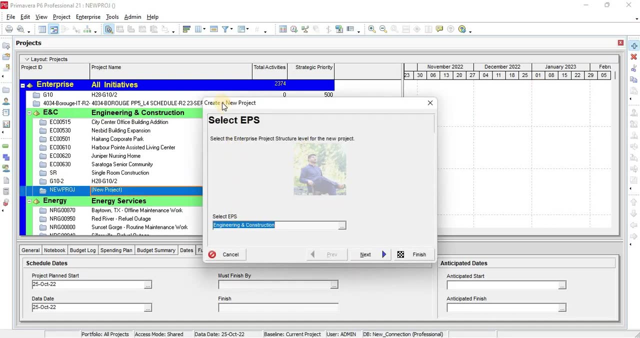 develop schedule for this layout. to develop schedule: now I am in the project window in Primavera. I will just simply click add. here we can see create a new project from the here I will define EPS for my project, in which department this project will exist for me. 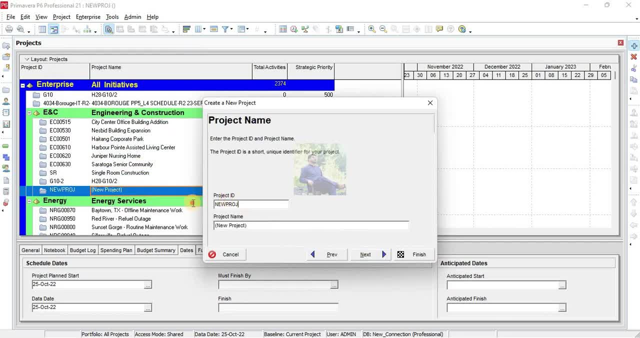 this engineering and construction project is okay now. 25 by 50, it is five. Marla house 100. I want to keep this my project ID and name of the project: 25 by 50 two-story house. this will be name of my project and start date. I want to start this project from first. 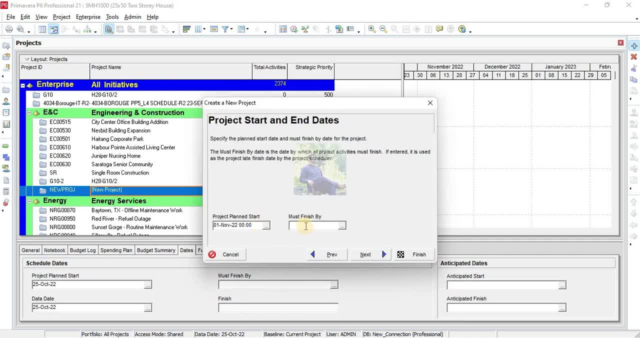 November 2022 and must finish date. I will leave it here because if I put some date here, this will create a constraint on my project, so I will leave this. one. responsible manager will be E&C manager is responsible for all the work in engineering and construction department, so my responsible 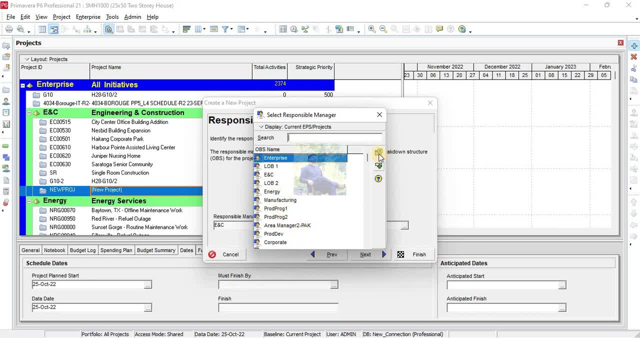 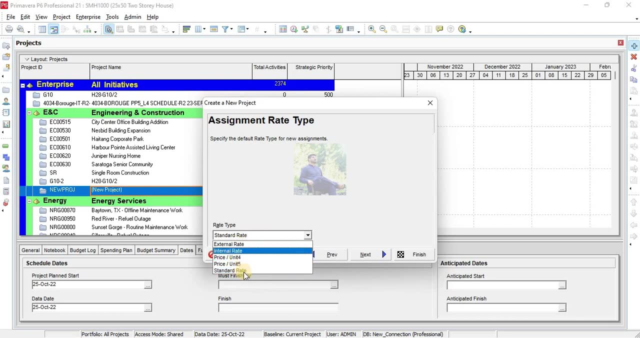 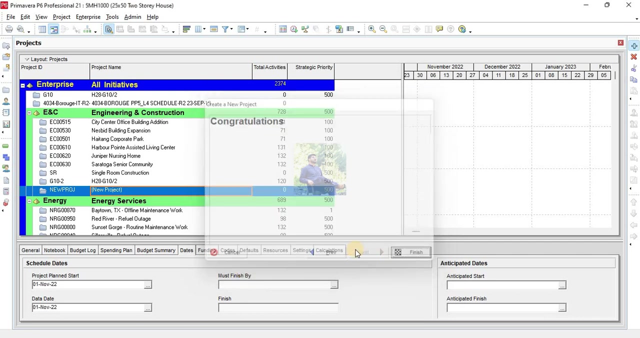 manager is E&C or you can change it from here, but E&C is okay for me. rate type: keep this standard rate type or you can change from here, but usually we do standard rate type. so my schedule is developed here. now I want to create WBS is to save time. I have already. 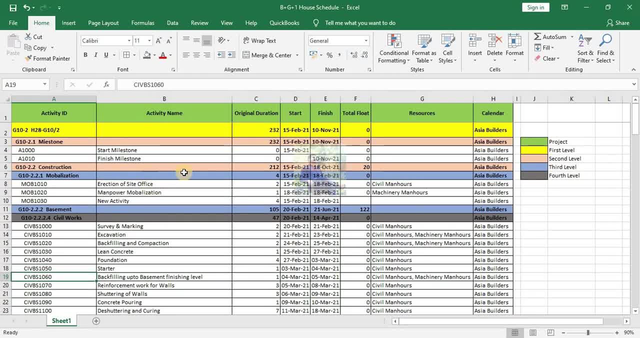 developed this schedule in Excel, so this one is project project. I have already defined first level milestone. this one is first level milestone. this one is first level milestone. this one is project project. I have already defined first level milestone. this one is first level milestone. this one is first level milestone. 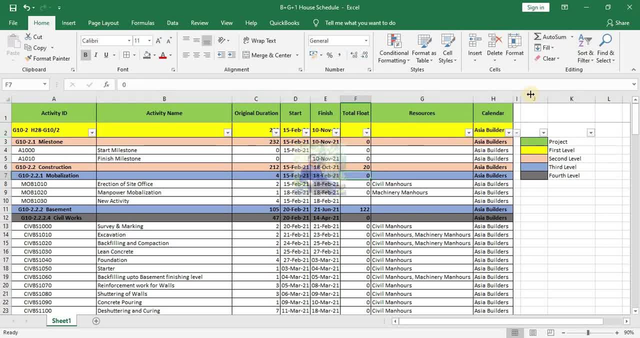 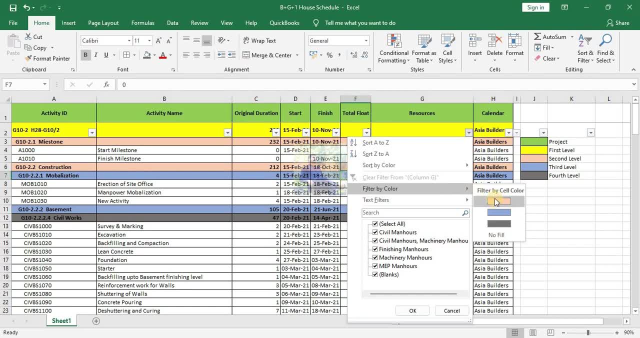 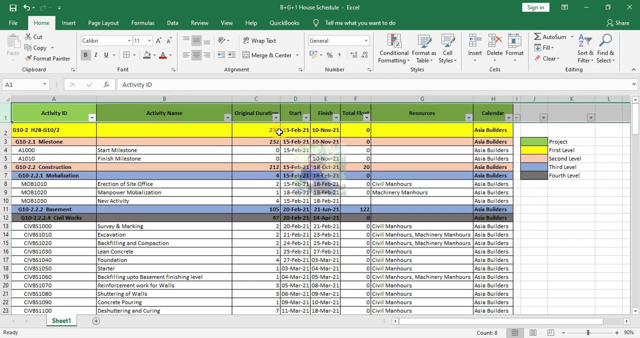 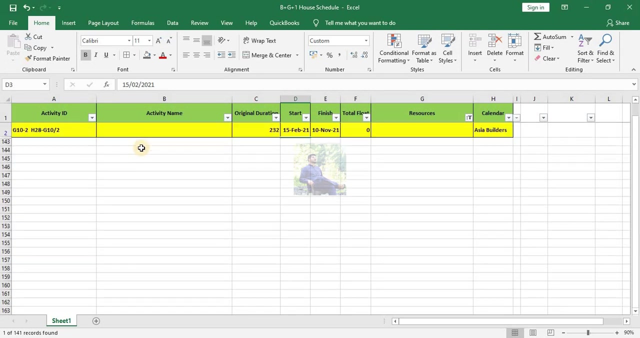 I want to create filter here and from here I want to filter by color. so filter I will add from here with primary. it is mandatory that you have in deep knowledge, knowledge of Excel also, so I will filter. so this one is first level milestone and 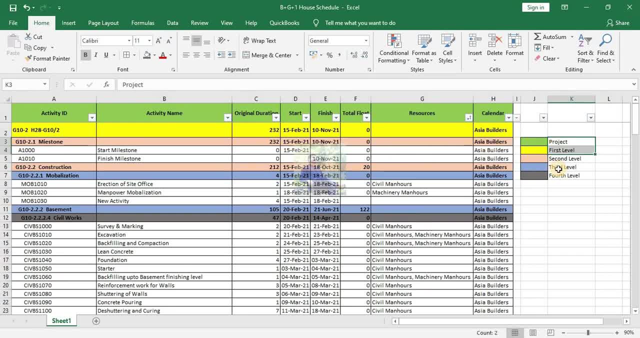 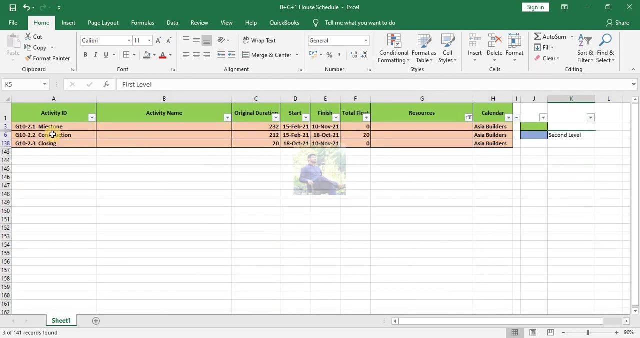 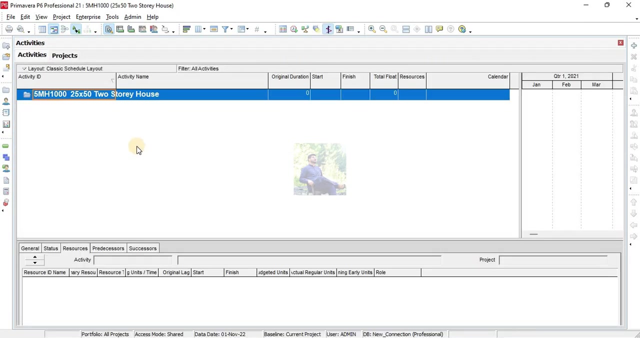 actually this one. I have defined one. so is project name. this is my first level milestone, so I will filter by color. this three are my first level milestone. now these I will define in Primavera will open this project. this is my project of five- marla house 1001, and project name is: 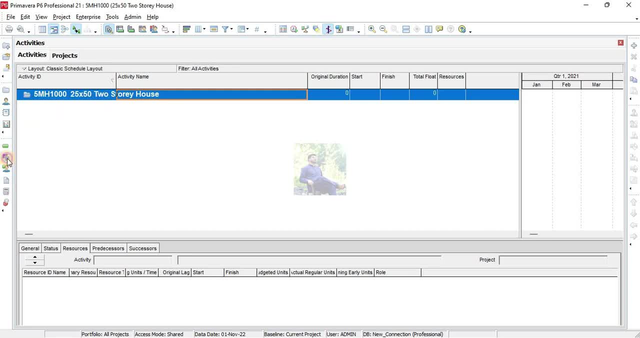 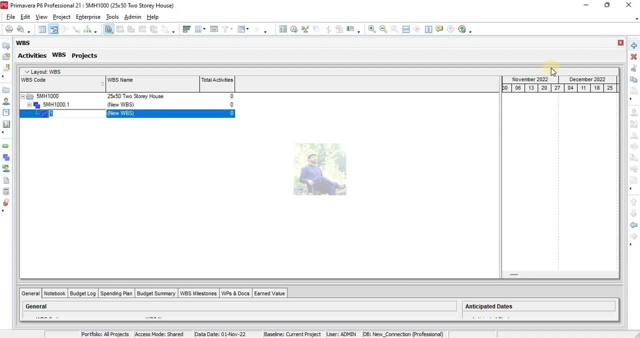 two-story house: 25 plus 52 two-story house. i will go to wbs window from here. you can go to wbs window on first level. there are three milestone. you can move milestone to left, right, up and down from from these buttons, from here milestone. 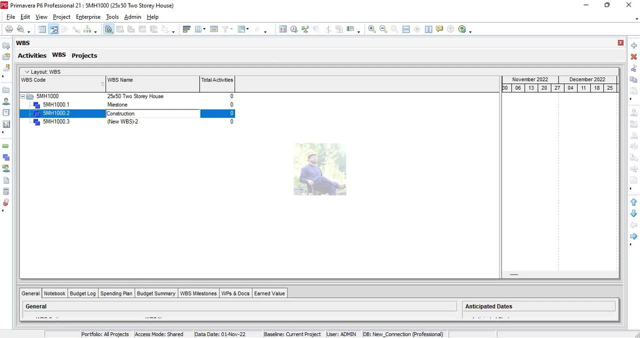 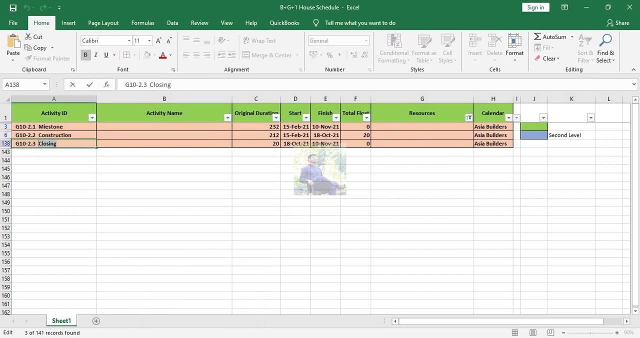 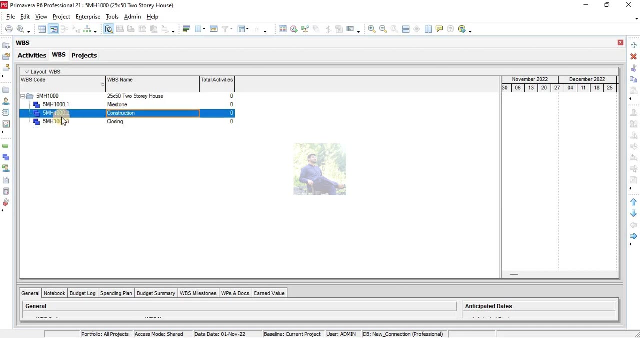 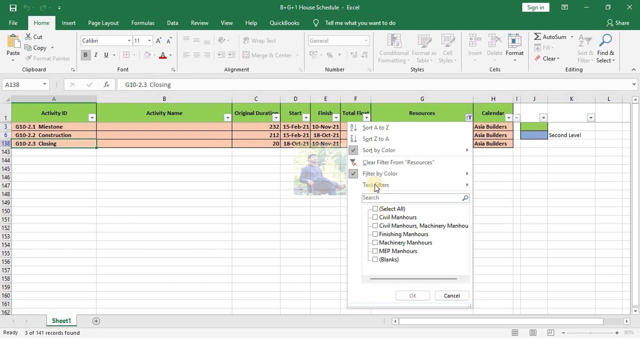 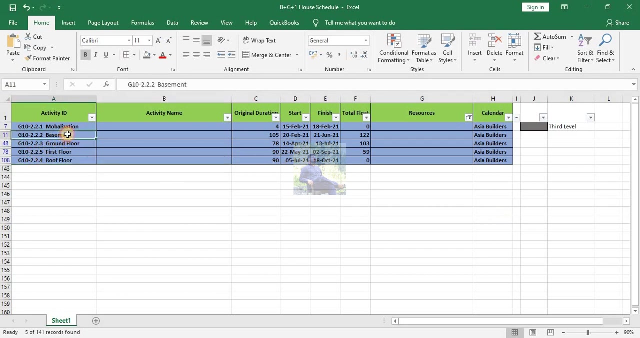 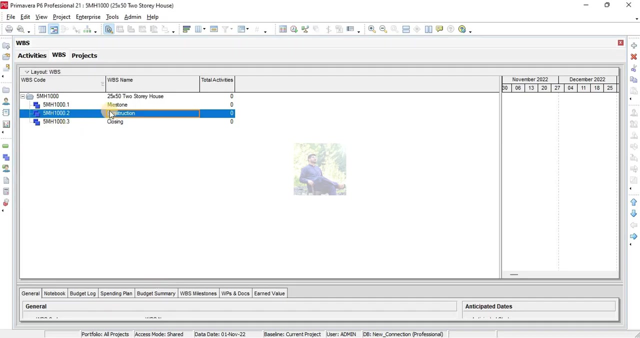 construction and closing. these are three first level milestone. sorry, wbs is now i will further divide these wbs's. in construction there will be mobilization basement. there is no basement in this house: ground floor, first floor and roof roof floor. so in construction there will be a mobilization ground floor, first floor and row floor. 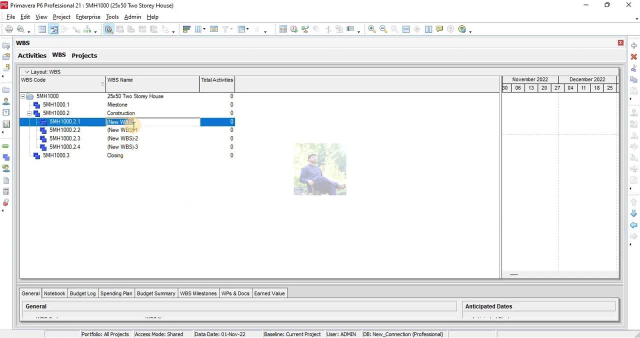 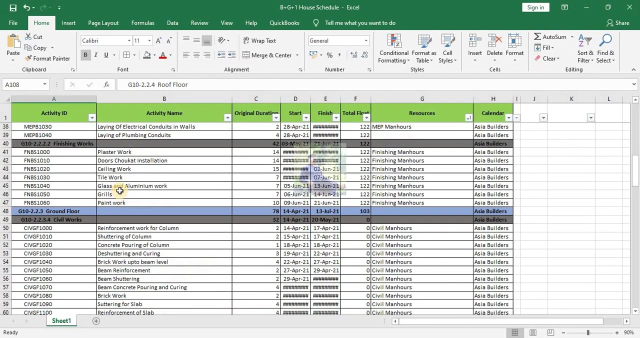 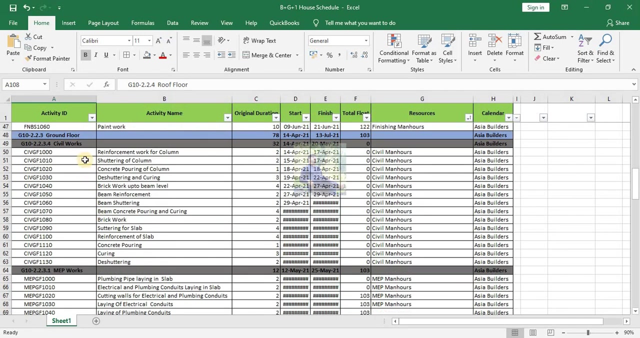 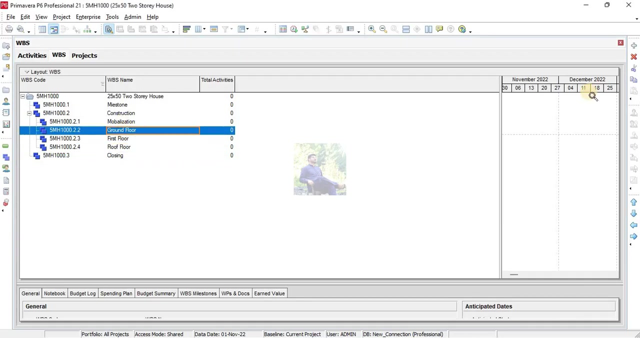 now moving on to the second level or and there is a personal City � itaaaaaaaaaa fsssssssssssss ssssssssssssss clear filters now in on each floor there will be further WBS is civil works MEP works and finishing works three WBS is on each floor so I will develop only one 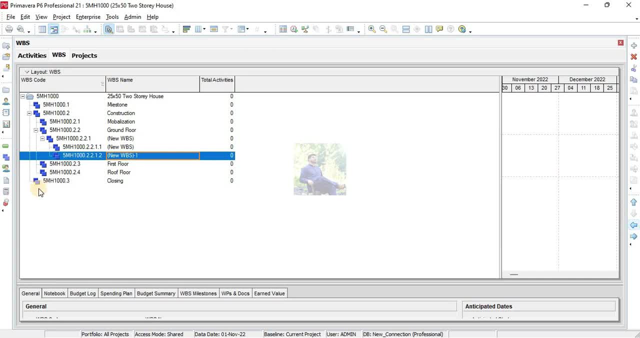 floor, WBS is civil works, MEP works and finishing works. these two floor I will leave it here. I will just copy WBS is and activities from ground floor because both will be similar to first floor and with minor changes to roof floor. also, I will just check closing and closing there is no. 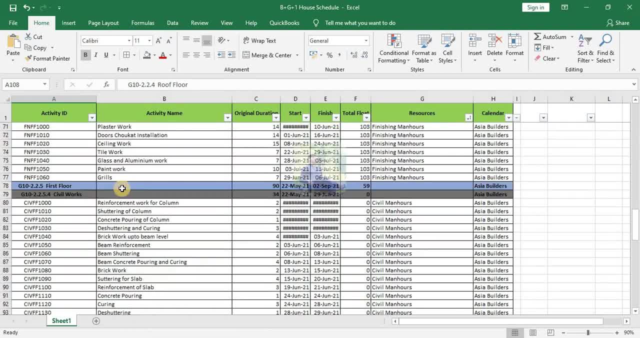 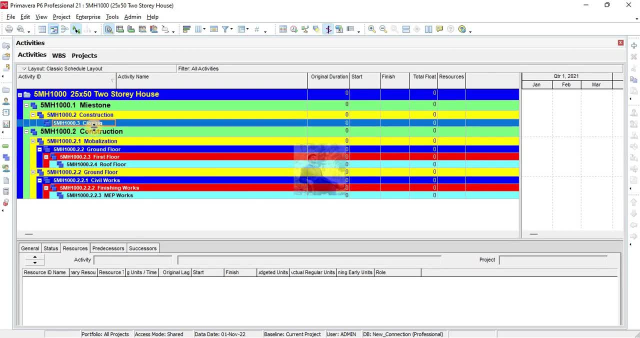 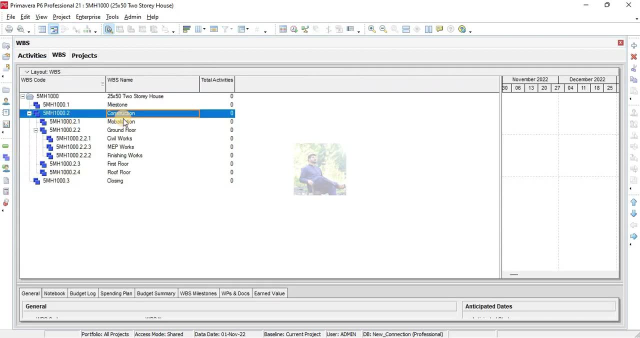 WBS. now I will come to activities. from here we can see that WBS is are shown in a wrong manner, because here you can see that under construction there is mobilization and underground floor there is civil works, MEP works and finishing works, but here it is not showing in the same manner to 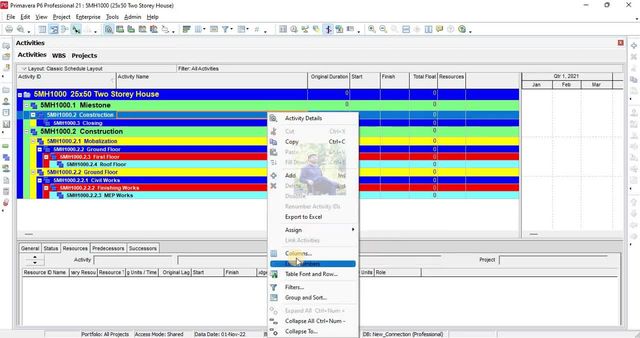 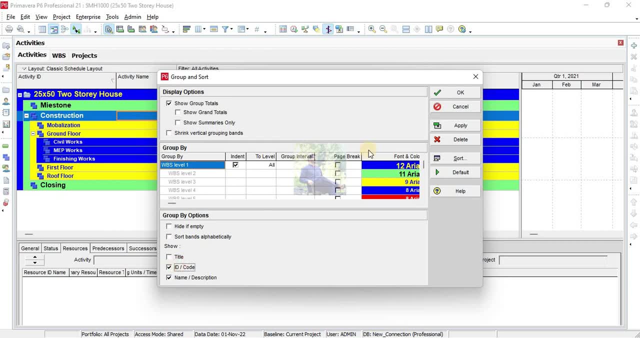 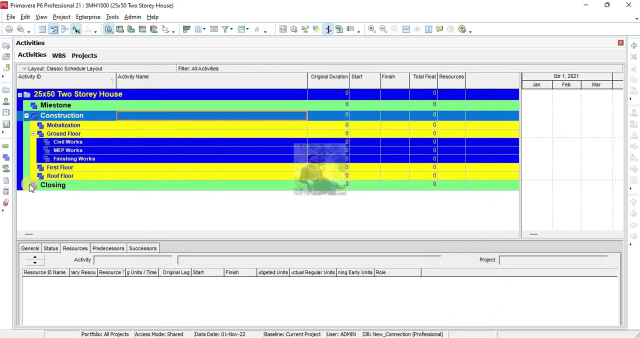 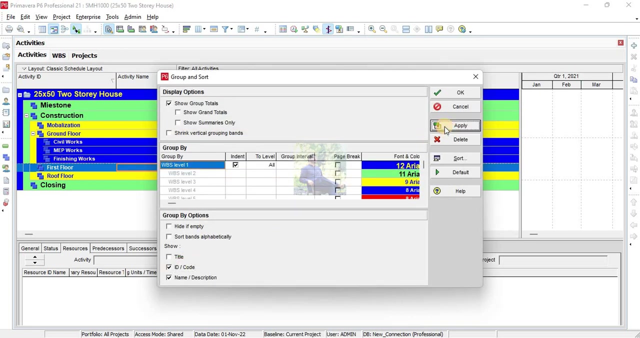 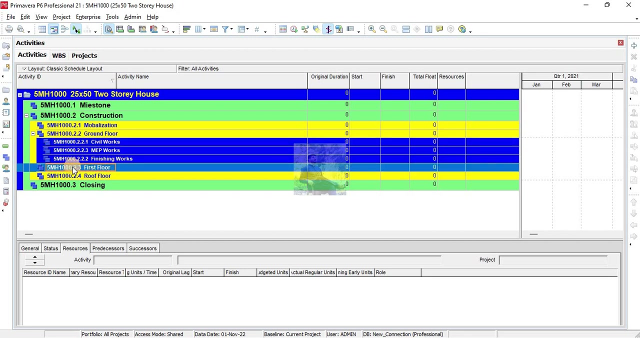 remove these bug. we will go to group and sort and I don't want to see ID code, so I just click here. or if you want to see ID code, you okay. now it is showing in in the same manner like in WBS window. now I will. 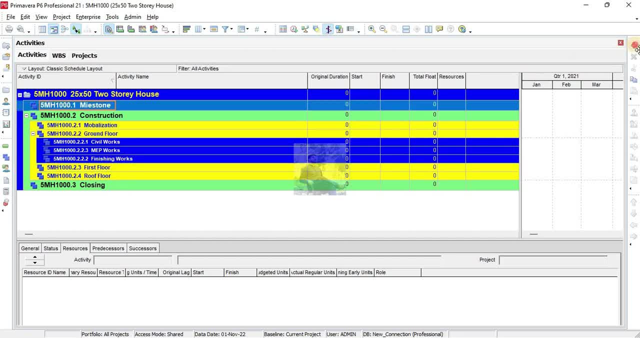 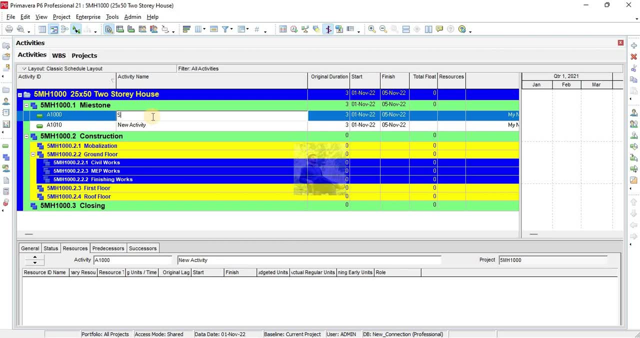 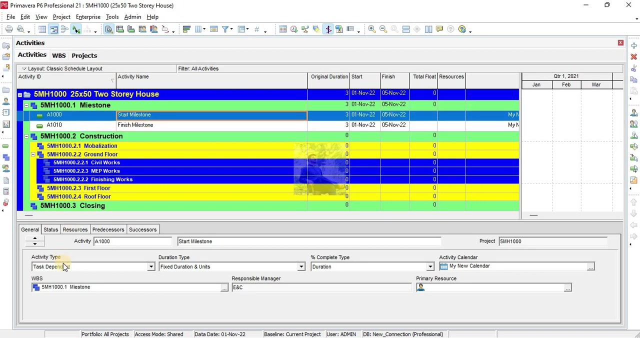 define activities in milestone. there will be two activities: start milestone and finish milestone. now, from general, you can see here that both of these activities are task dependent, so we will just change it to start milestone and this one to finish milestone. so these two activities are defined and now I will come to construction. in construction, in mobilization, 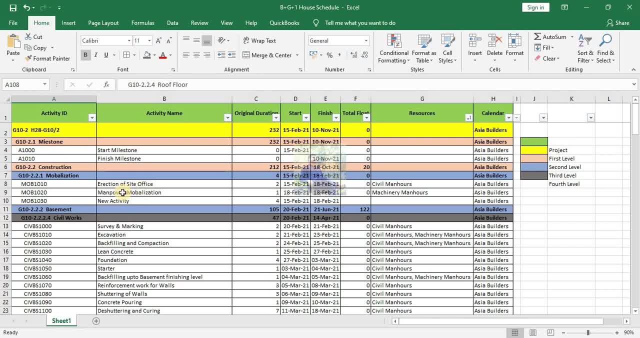 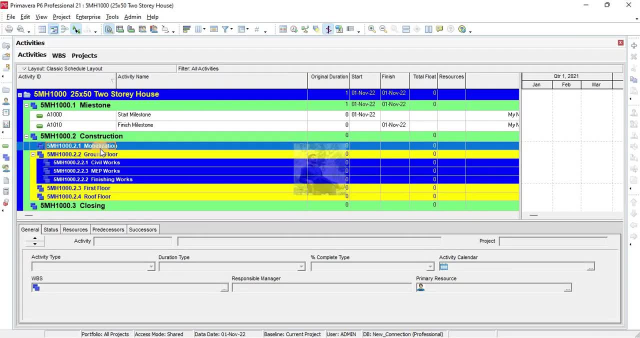 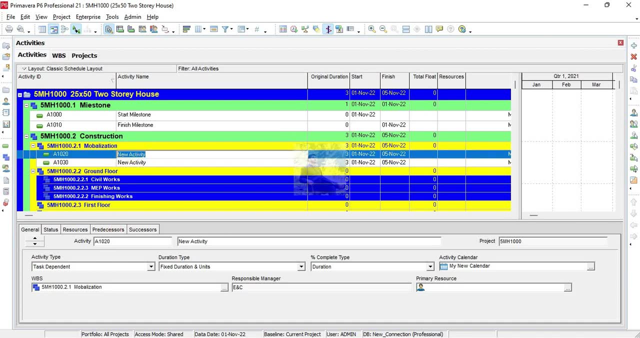 from here. I will just copy the activities. in mobilization there will be erection of site office and manpower mobilization. in mobilization there are two activities I will just copy from here: okay, okay, erection of site office and manpower mobilization. so these two activities are defined. now I 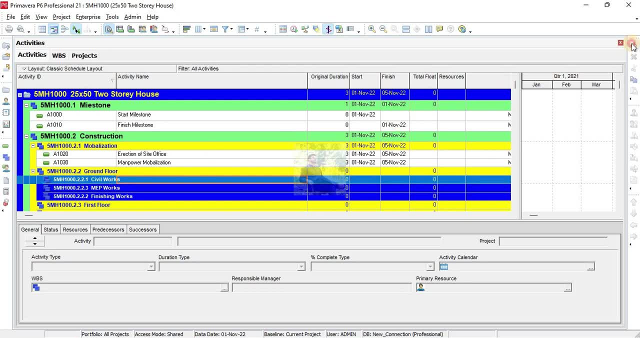 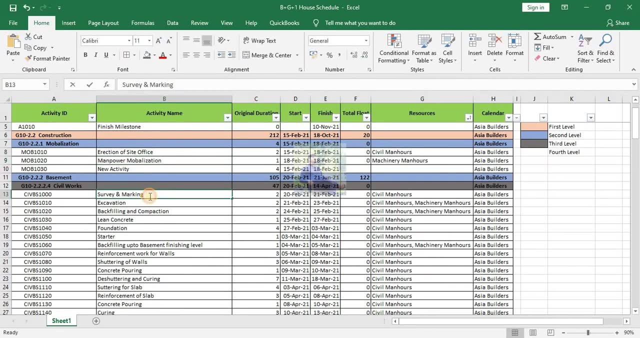 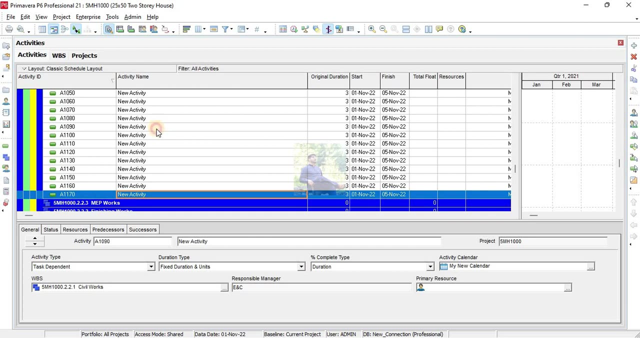 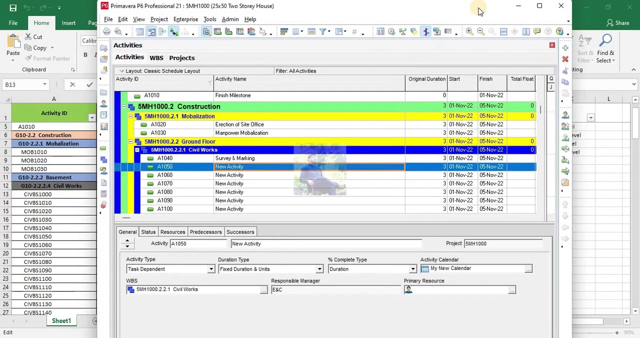 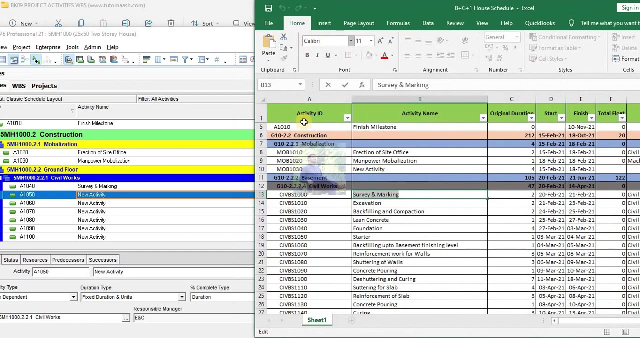 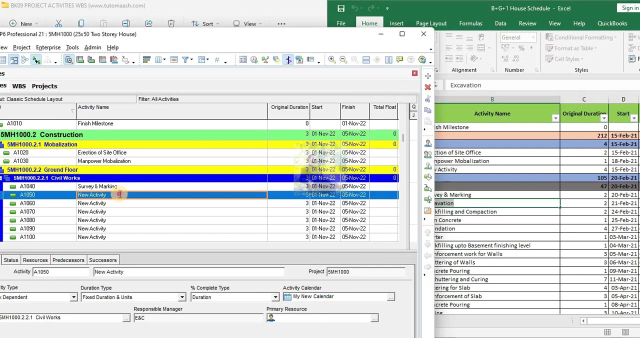 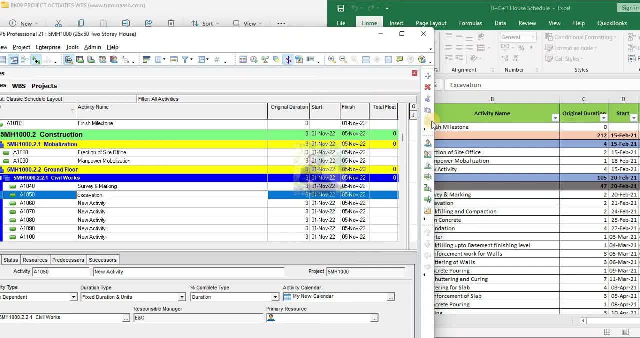 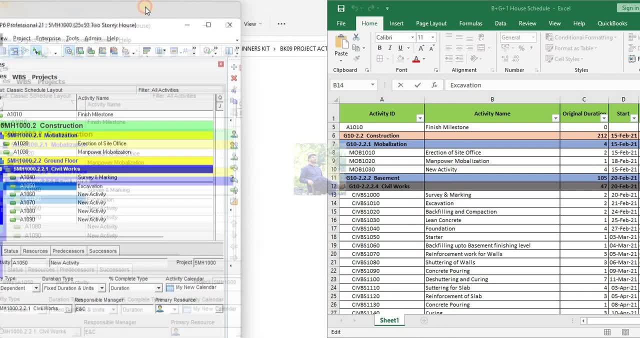 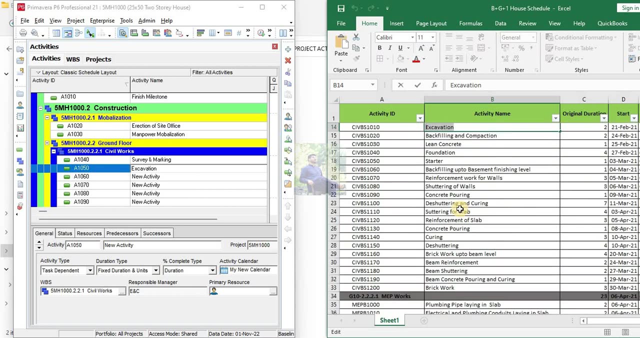 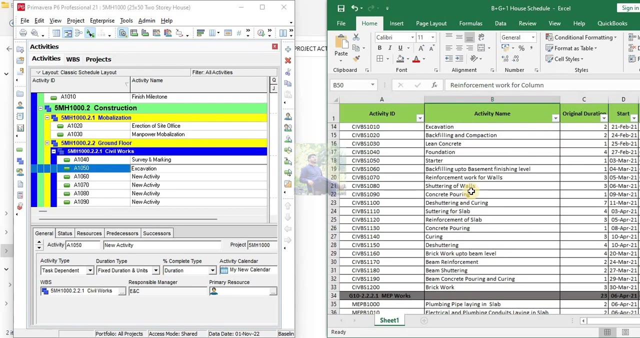 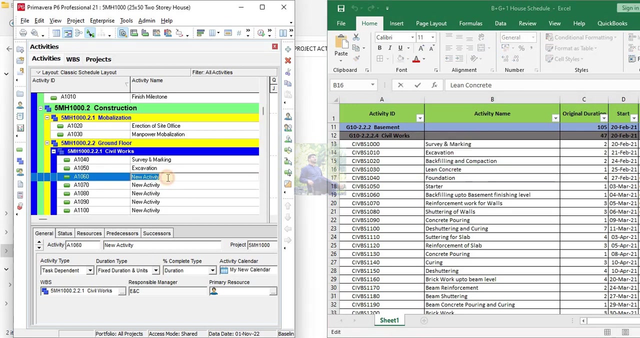 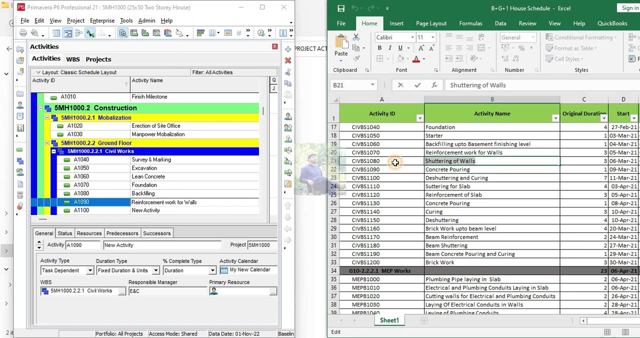 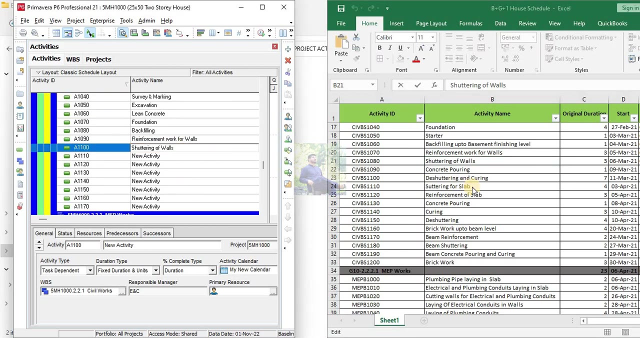 okay, then I welcome to ground floor excavation. then there will be lean concrete, then foundation after foundation, then there will be back filling, if required, and after back-filling, reinforcement: reinforcement of walls, shattering of wall, concrete pouring of walls, then de-shattering of walls, then de-shattering of walls. 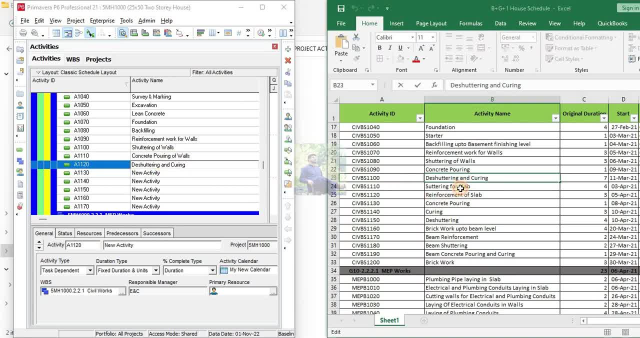 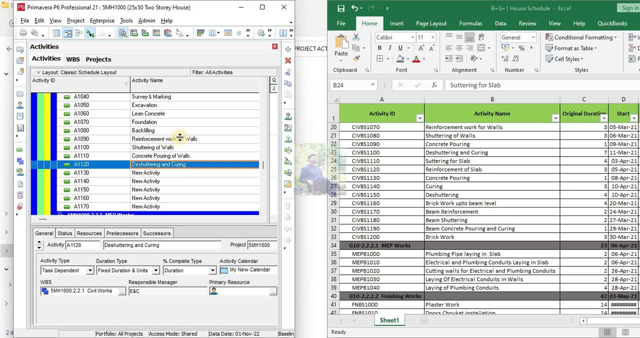 and curing this will be of walls, and and curing this will be of walls, and and curing this will be of walls and columns. if there is some brickwork, we will. if there is some brickwork, we will include in same. include in same. then there is a shuttering of slab. 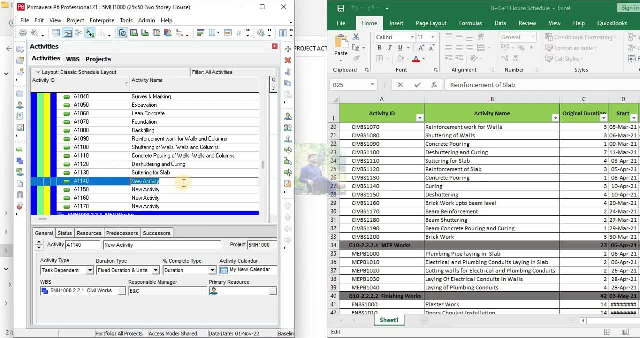 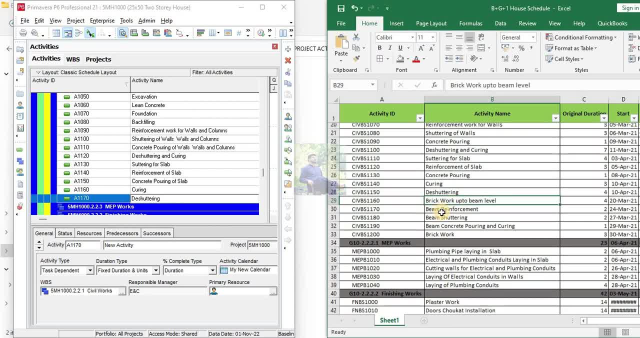 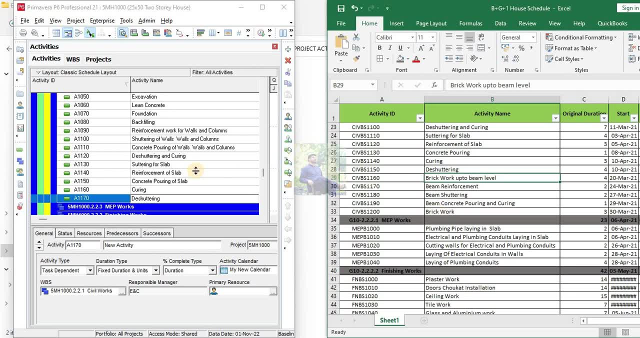 de-shattering. so what we have to do is here, i have developed this schedule. i here, i have developed this schedule. i here, i have developed this schedule. i have have have made brickwork in a separate activity, made brickwork in a separate activity, made brickwork in a separate activity. so from here. 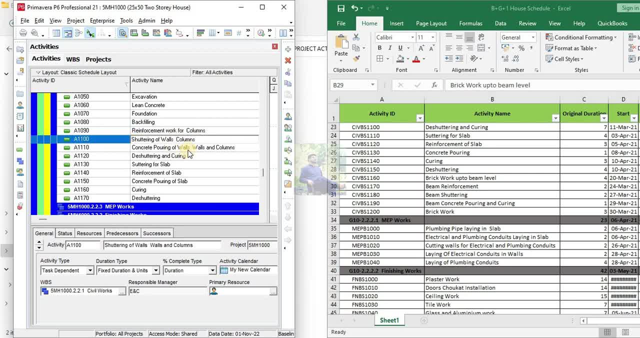 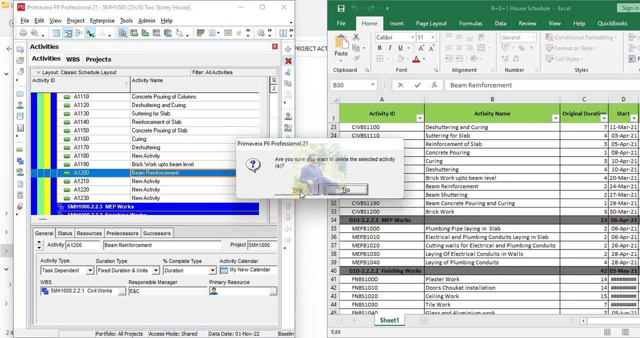 i will delete this one. i will delete this one. brickwork up to beam level or lentil beam. brickwork up to beam level or lentil beam. brickwork up to beam level or lentil beam, or I will just delete this activity and brickwork in ground floor. okay, so 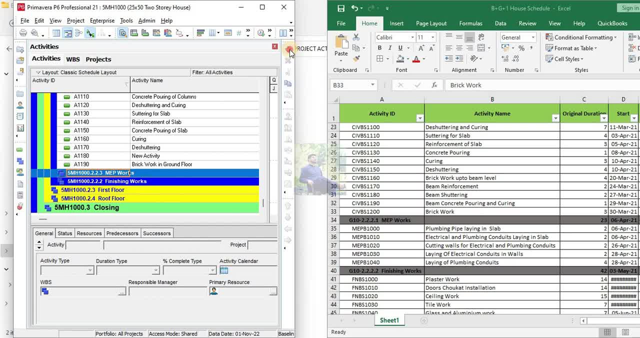 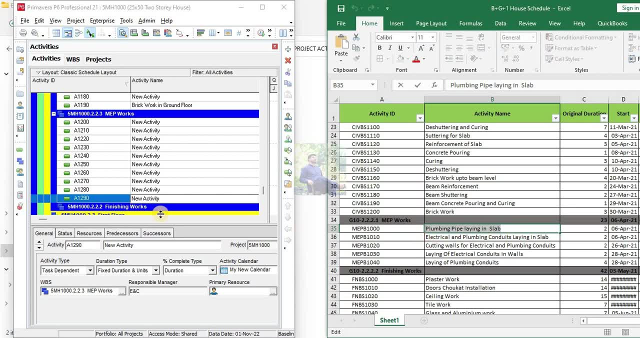 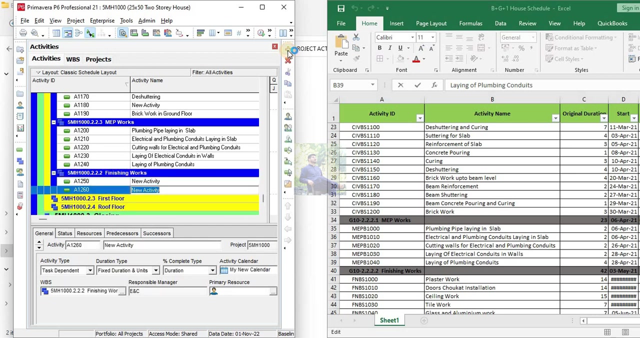 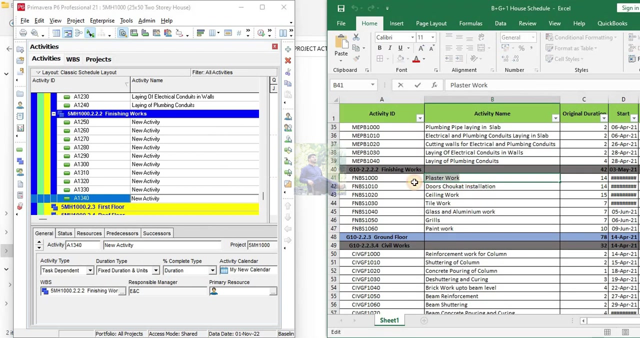 now I will come to MEP duties. same. I will copy from here length of electrical cables and finishing work. in finishing work there will be plus: Master work, Doors and Chalket Installation, Ceiling Work, Tile Work, Glass and Aluminium Installation, Grill Installation, Paint Work, Ceiling Work, Ceiling Work. 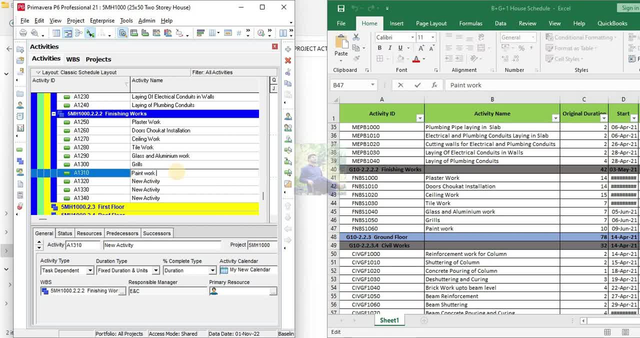 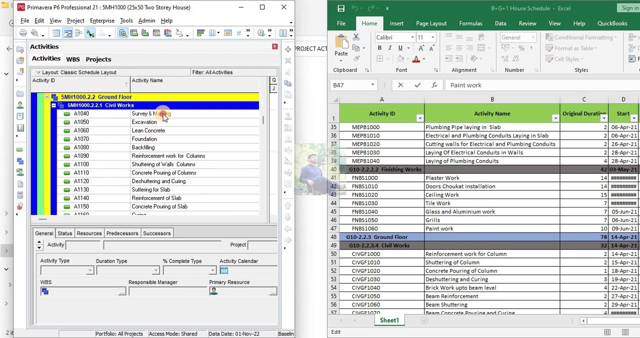 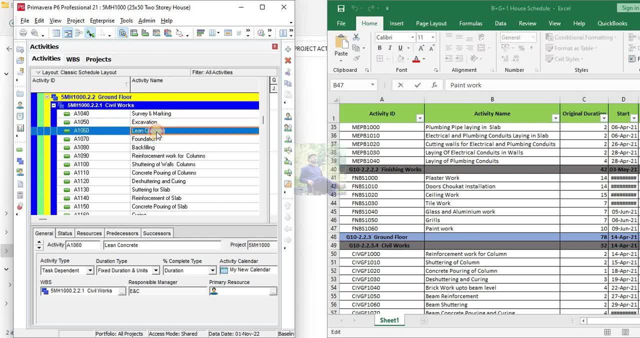 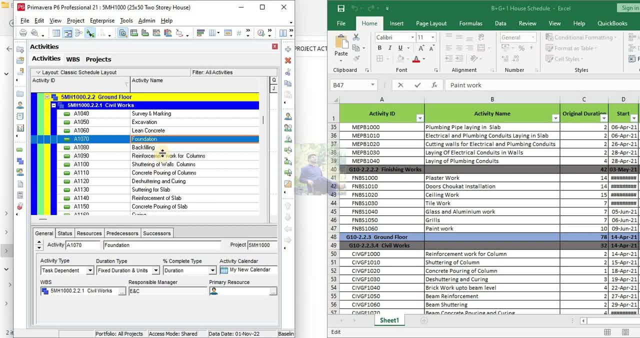 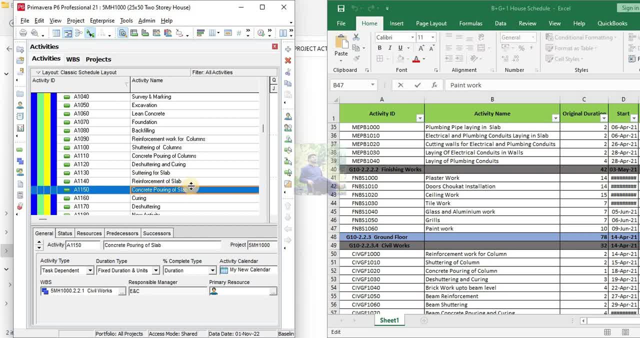 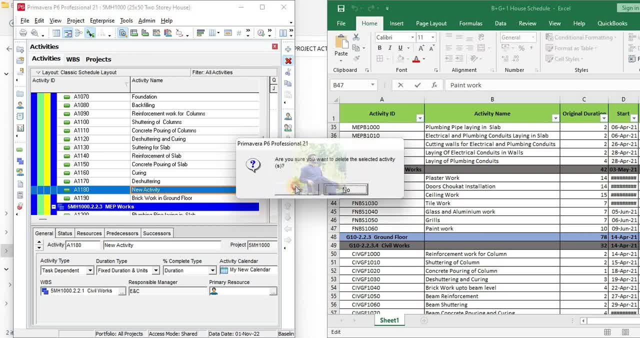 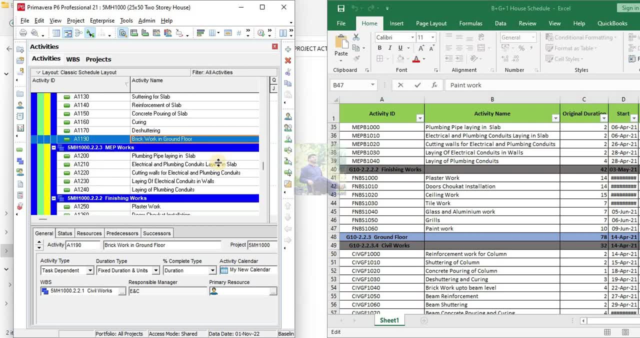 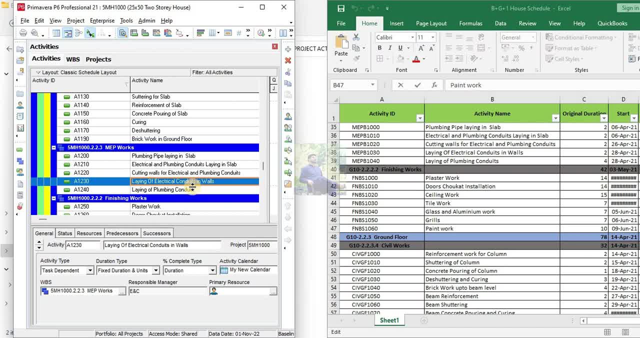 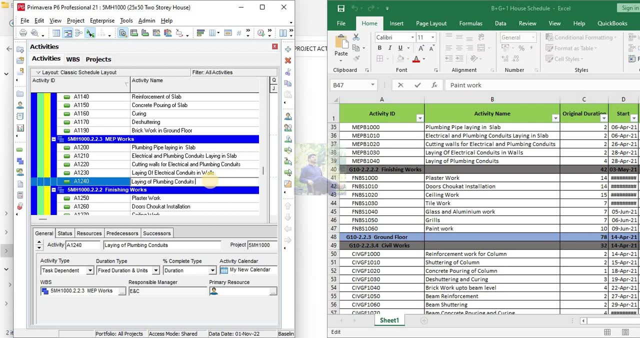 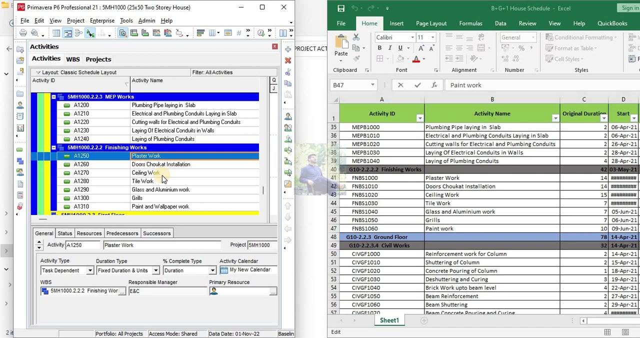 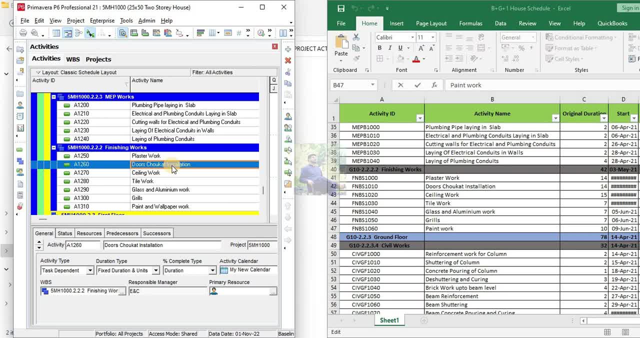 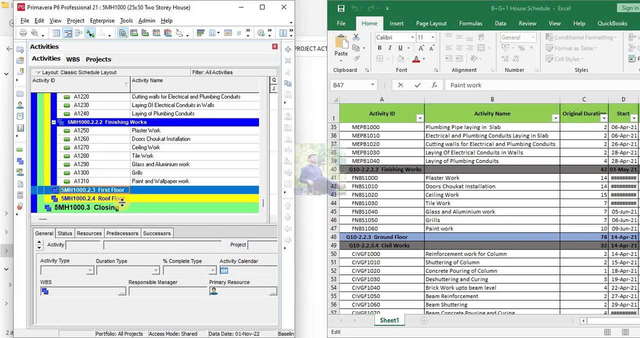 work. after ceiling work is completed we will do tile work. many people do tile work before ceiling work, then after tile work there will be glass and aluminum work and grill work and after last there will be paint and wallpaper work. first floor activities will be same, so now I will not copy these activities now. 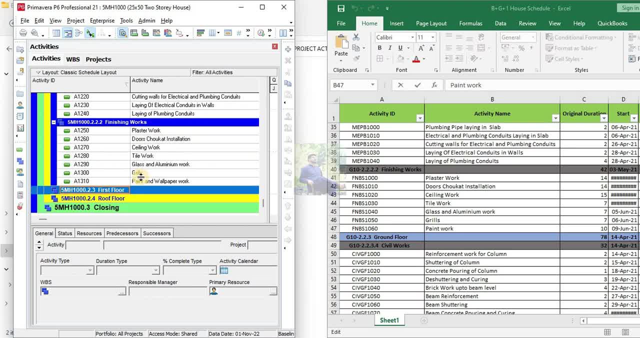 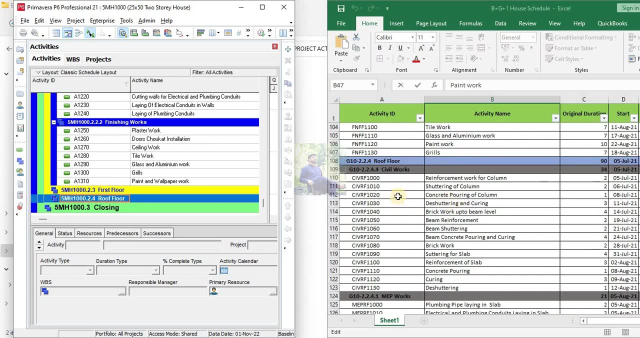 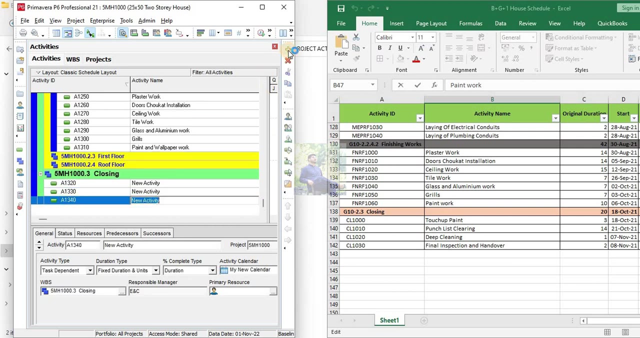 into first floor. first I will sequence these activities for duration there. then I will copy it. now I will come to roof floor. in fact in row floor activities will be same and in closing there will be touch up and then there will be punch list clearance and after punchless punch list clearance there. 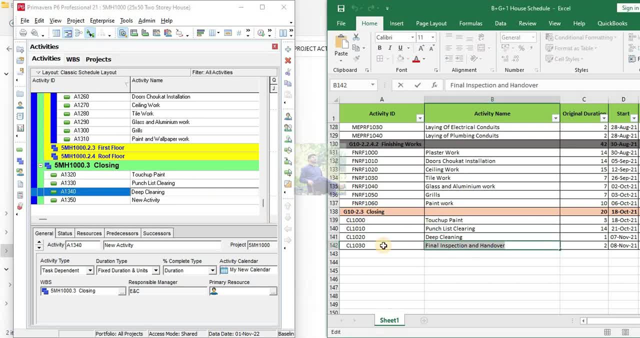 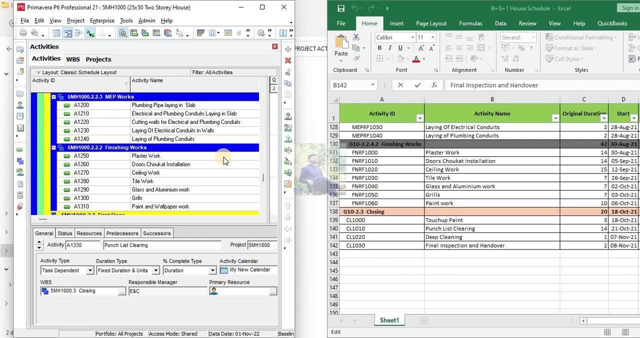 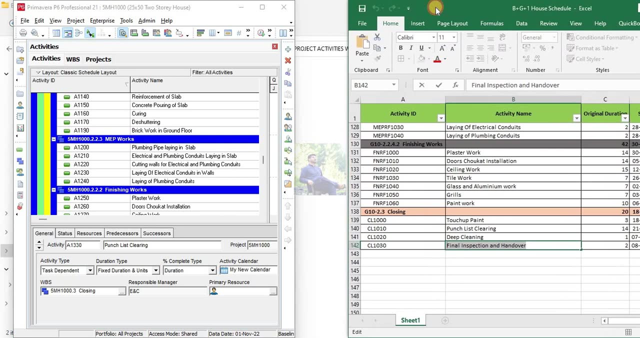 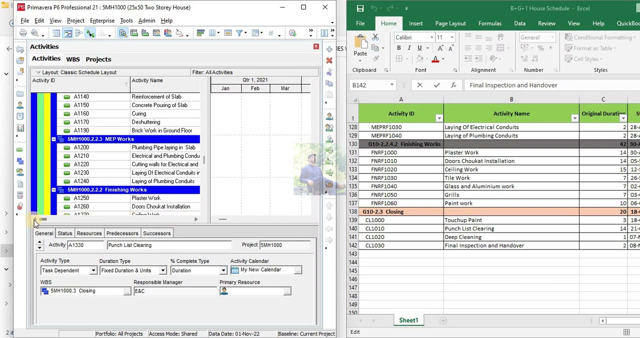 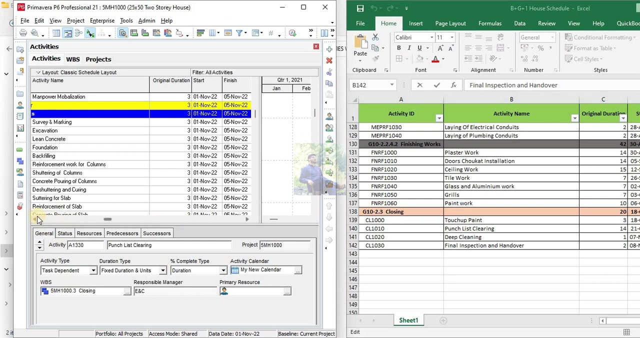 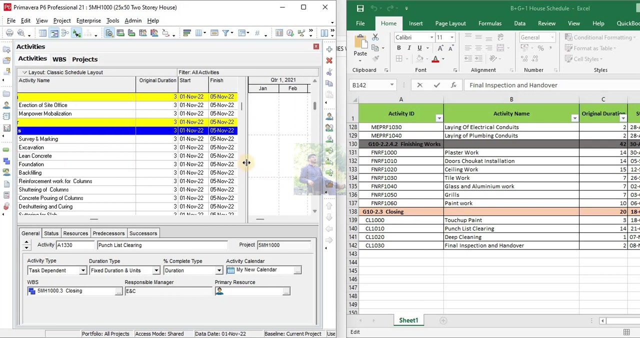 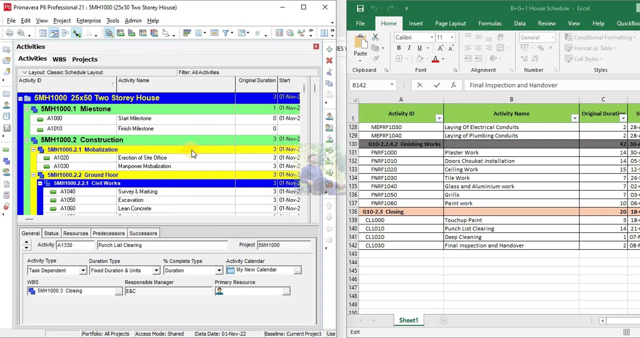 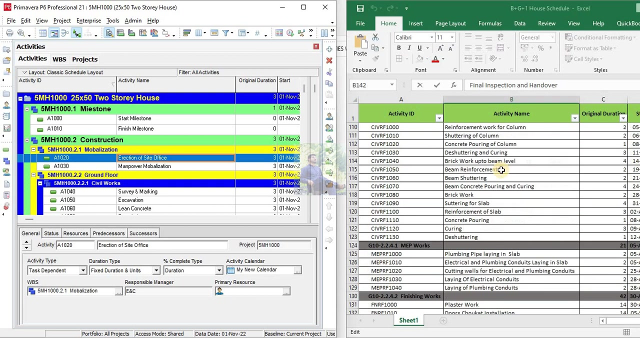 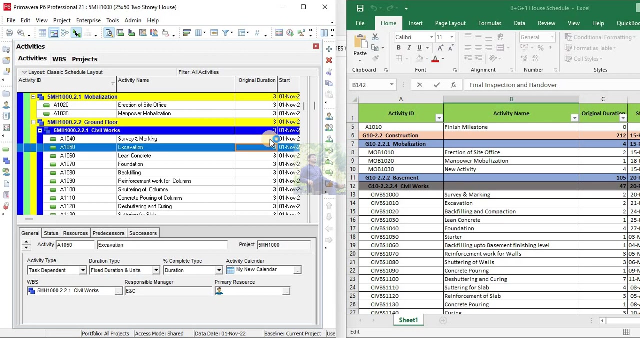 will be deep cleaning of the house and after deep cleaning, final inspection and handover now. after that I will assign durations and make this column smaller. so definitely start and finish. milestones have zero duration from here. I will start: survey is having two days, then excavation: two days for excavation. 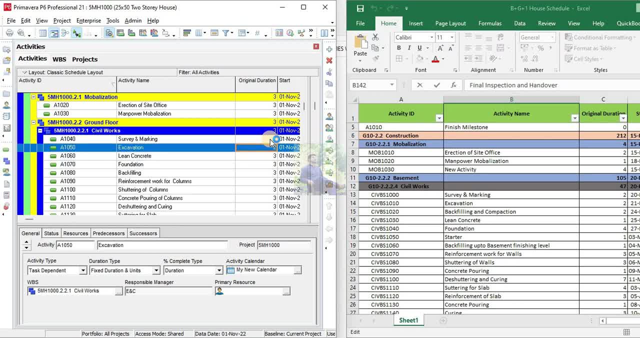 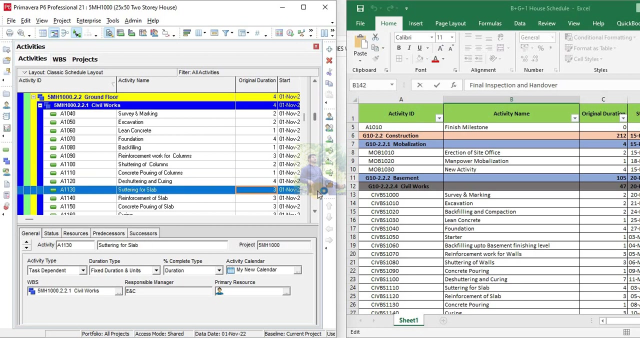 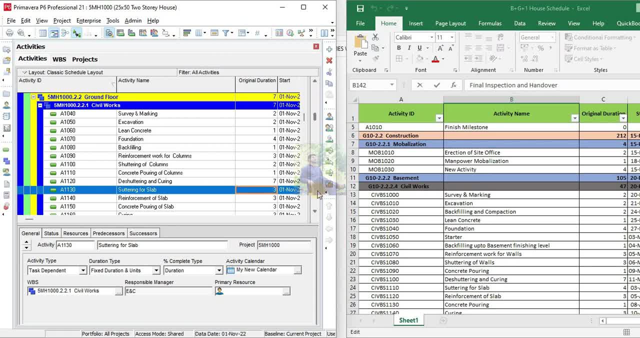 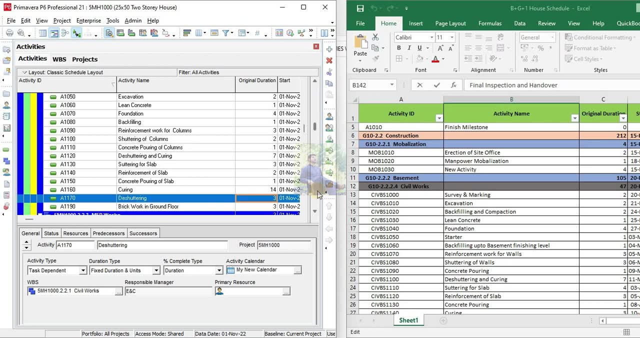 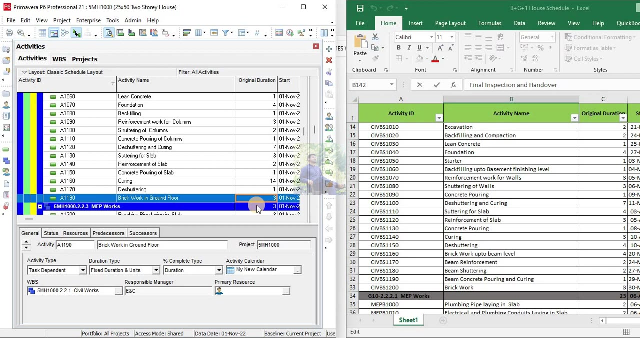 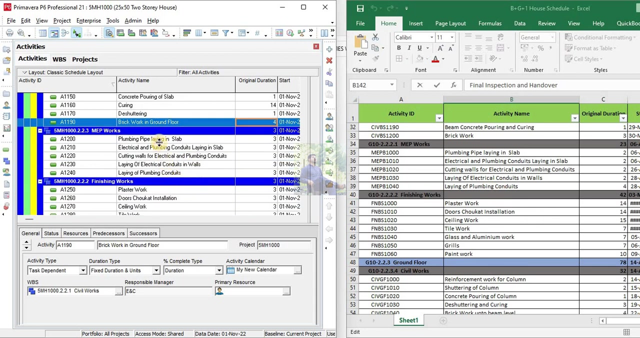 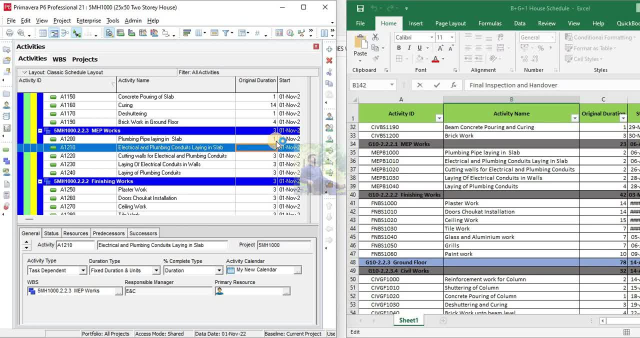 plumbing pipes in slab. electrical pipe laying in slab: this will take one day. cutting walls, this will take one day. laying of electrical conduits in wall, this will take one day. and laying of plumbing conduits: this will take one day. cluster work will take, let's say, five. 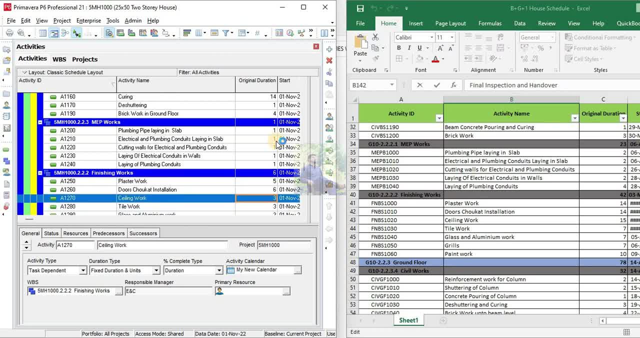 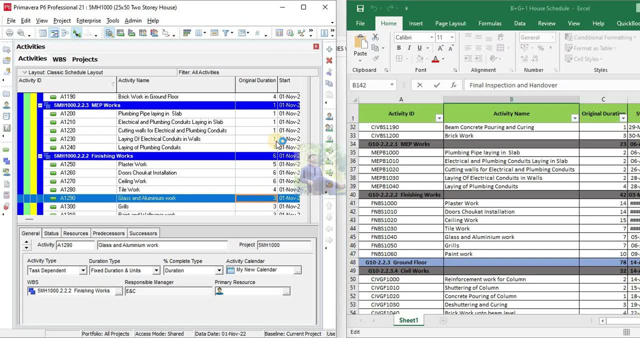 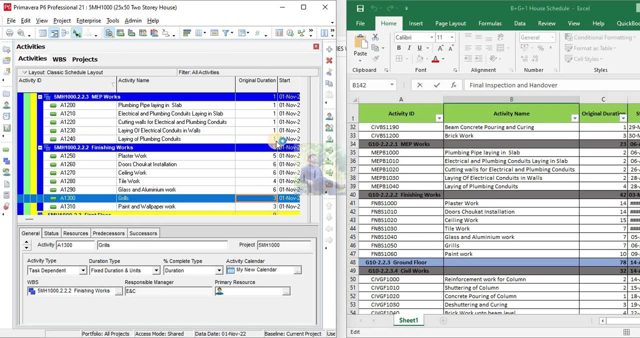 days. doors and chocket installation six days, ceiling work six days, tile work four days and glass and aluminium work six days, grills two days and paint and wallpaper work seven days. by the way, this duration you have to put from productivity sheets. your company must have productivity sheets like one mason and one helper can do an average 20. 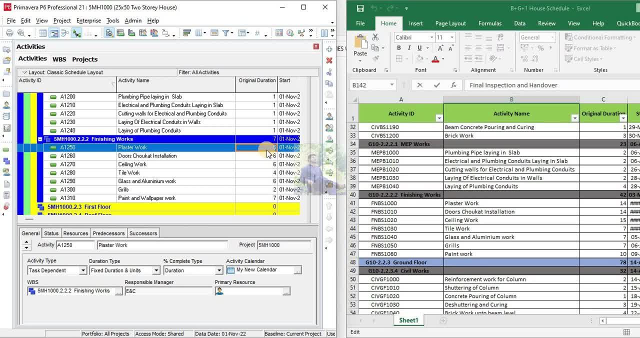 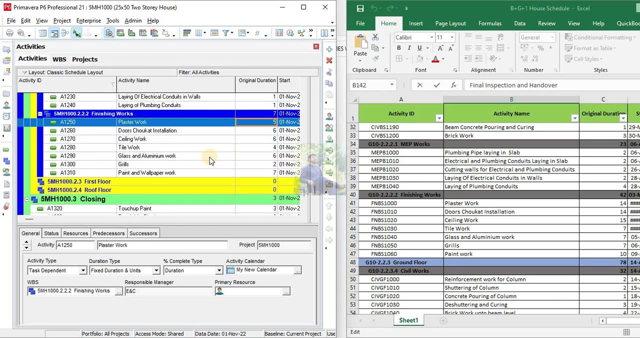 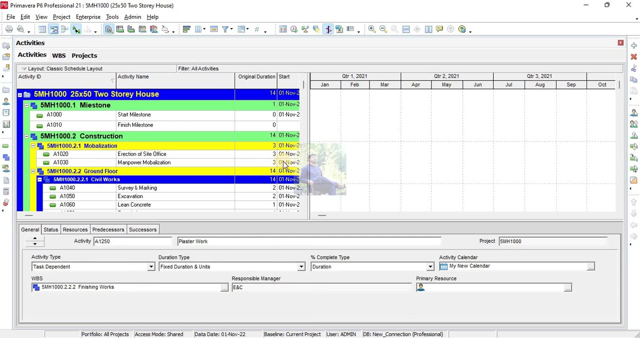 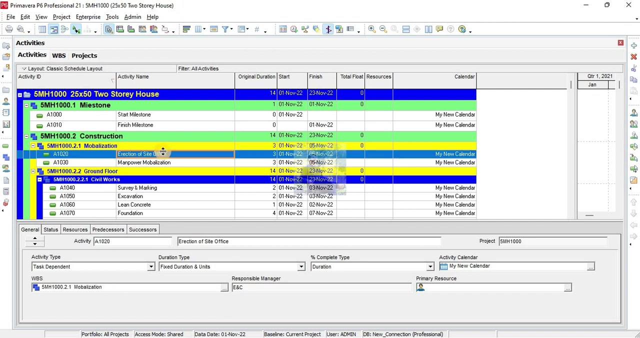 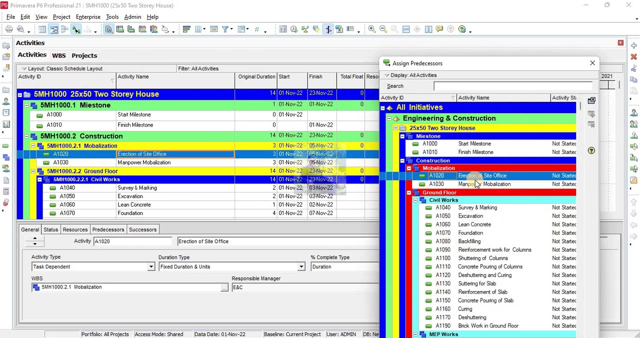 meter of plaster. so you will take duration from that productivity sheet, how many mason you have and how many area you have for plaster. from there you can calculate durations. now, what we have, we will do. I will sequence activities to sequence activities. assigned predecessors: erection of site from. 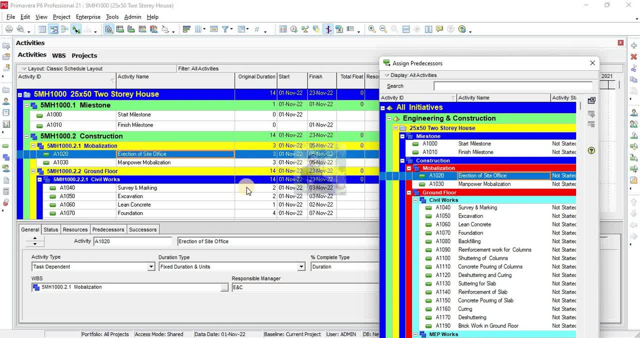 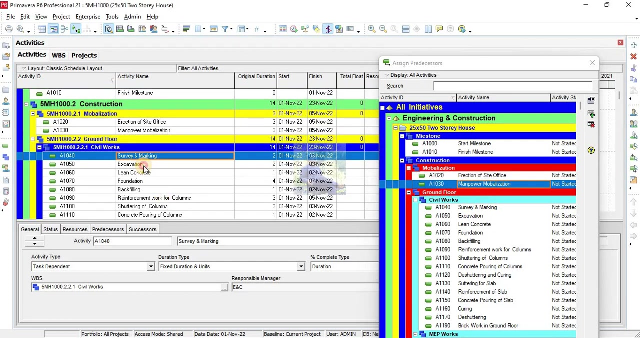 mobilization, my project will be started. so predecessors of this activity will be start milestone, then manpower mobilization. predecessor will be erection of site, then survey and marking. predecessor will be manpower mobilization. after survey and marking activity will be excavated, excavation and after excavation activity will be lean concrete, after lean concrete activity. 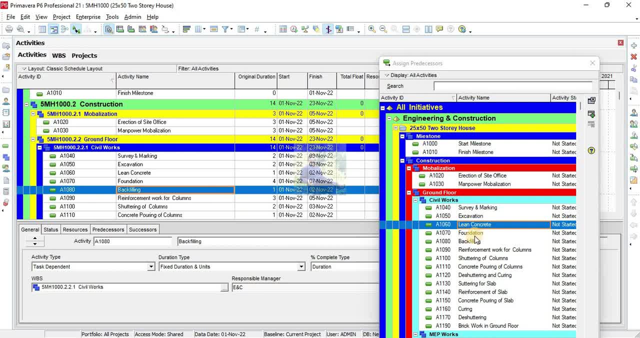 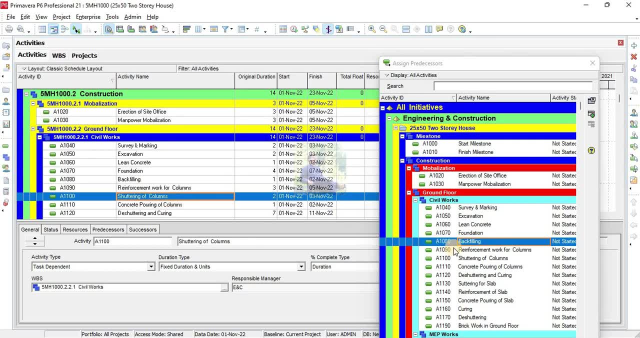 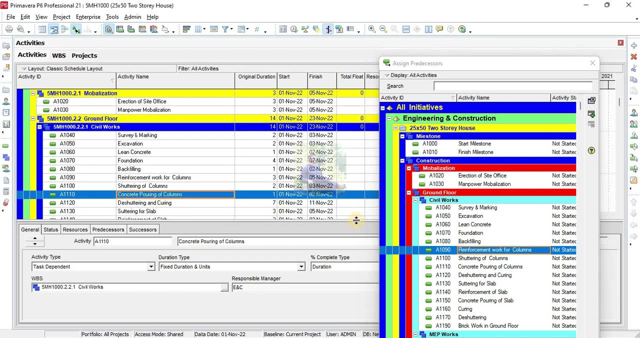 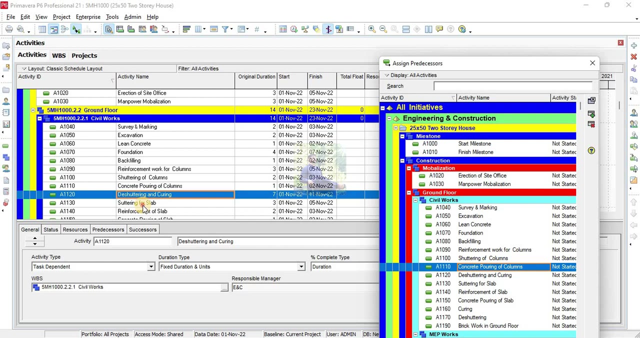 will be foundation and after foundation, activity will be big filling and after big filling activity will be the reinforcement of columns and after reinforcement of column activity will be shuttering of columns and after shuttering it will be concrete pouring and after concrete pouring, activity will be de shuttering and after de shuttering. 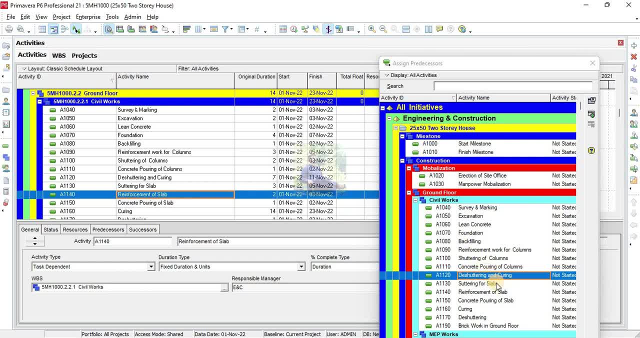 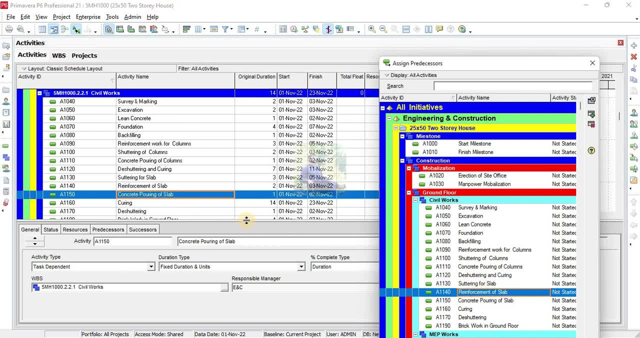 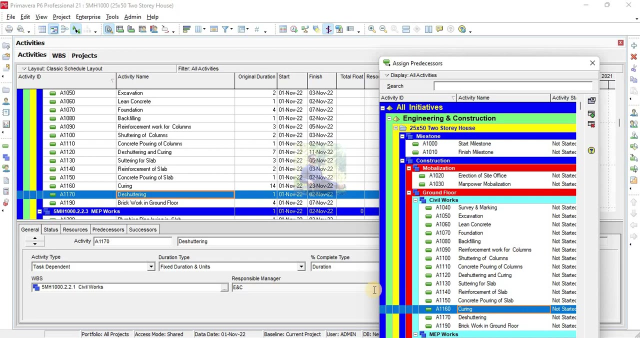 activity will be shuttering of slab, and after shuttering of slab we will do reinforcement of slab, and after reinforcement of slab we will do after reinforcement of slab we will do concrete pouring, and after concrete pouring we will do curing. and after curing we will do deshuttering. and after 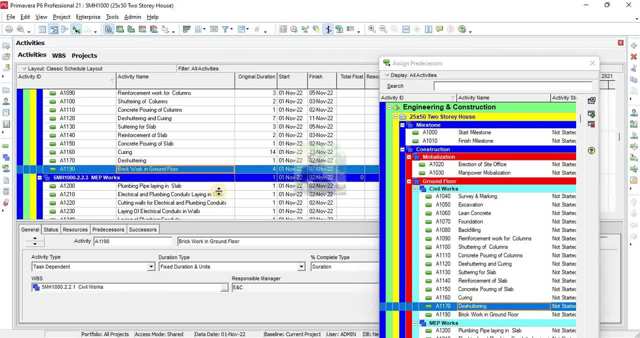 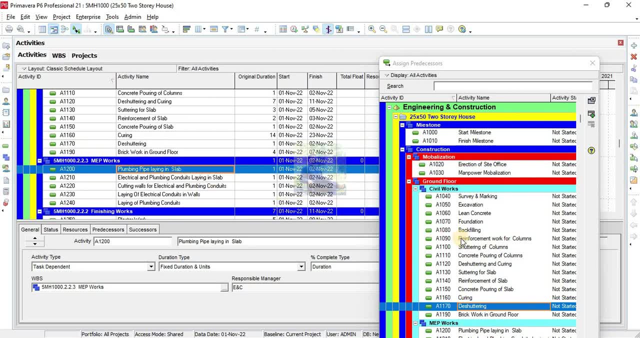 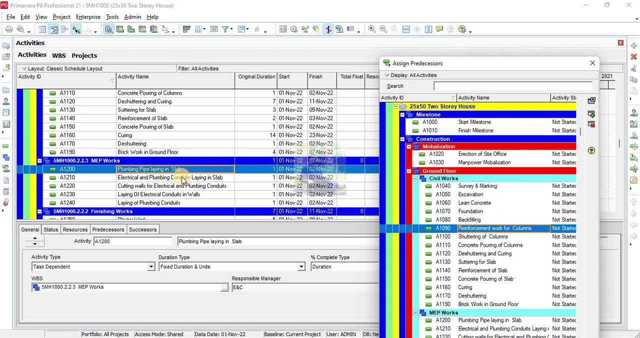 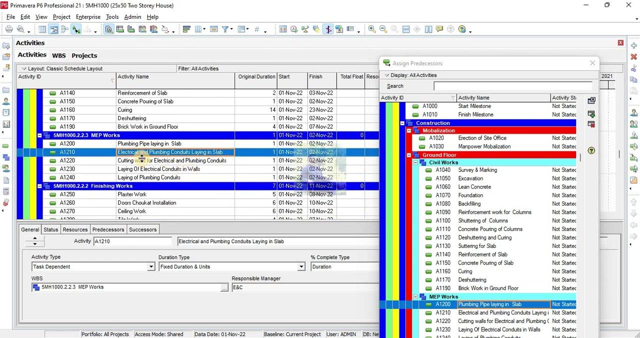 de shuttering, we will do brickwork, this plumping of pipe laying the predecessor of the lathe. this will be a reinforcement of column and for electrical and plumbing conduits, predecessor will be. in fact, this should be electrical conduits only cutting of walls. for this predecessor should be: 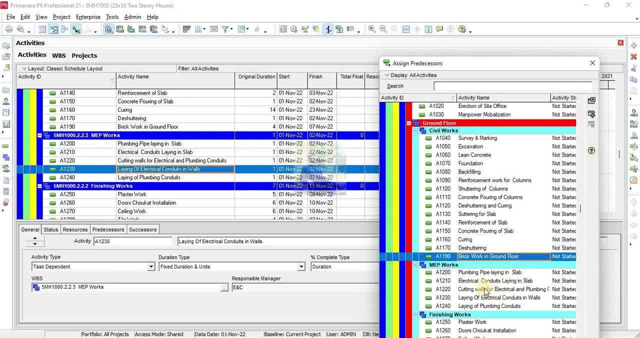 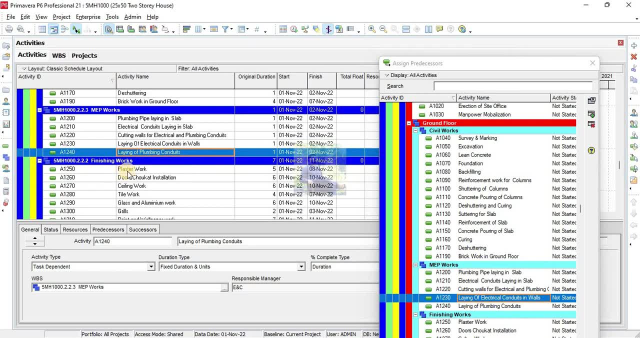 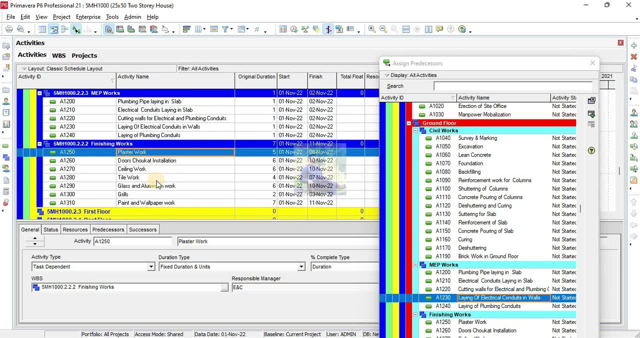 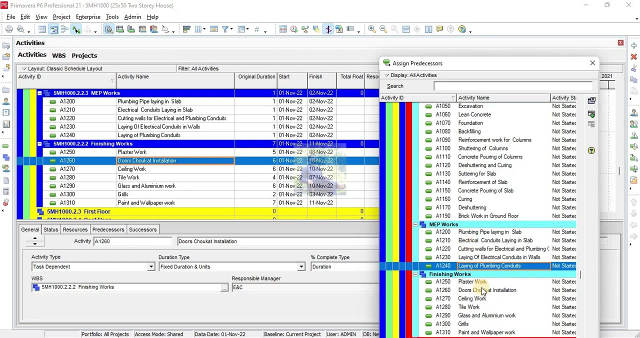 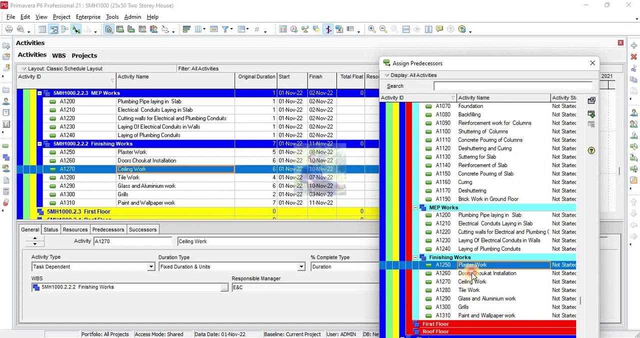 brickwork length for this predecessor should be, and for this predecessor should be this one. and plaster work predecessor should be this one and for this predecessor should be this one. and for ceiling work predecessor should be this one, and for tile work predecessor should be this one, and for glass work predecessor should be this one. and. 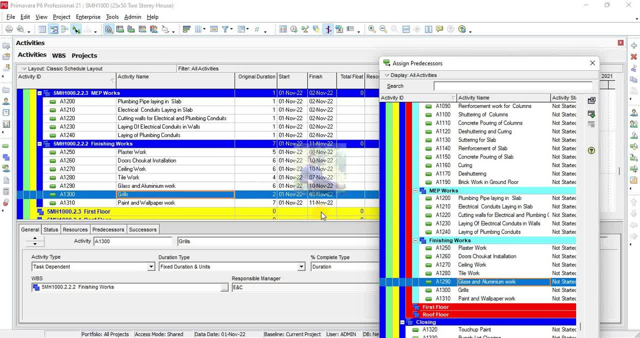 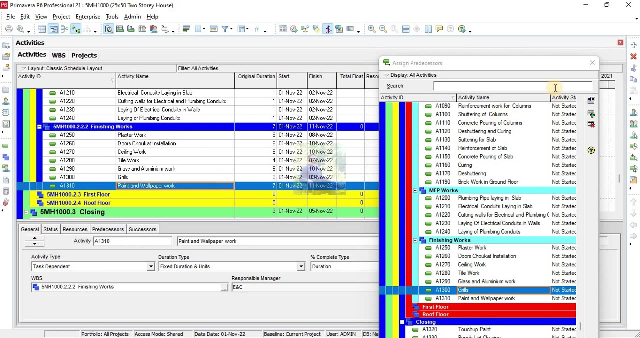 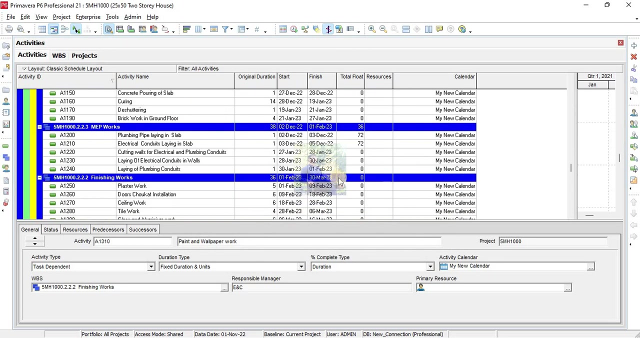 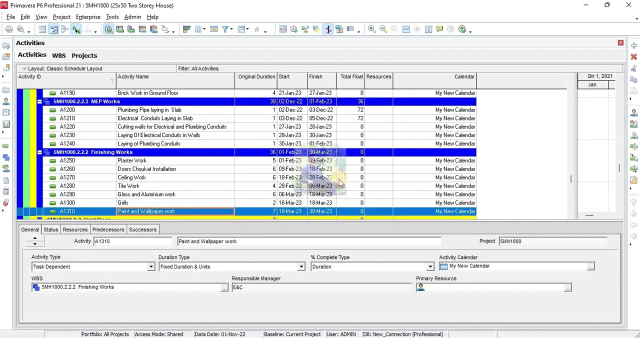 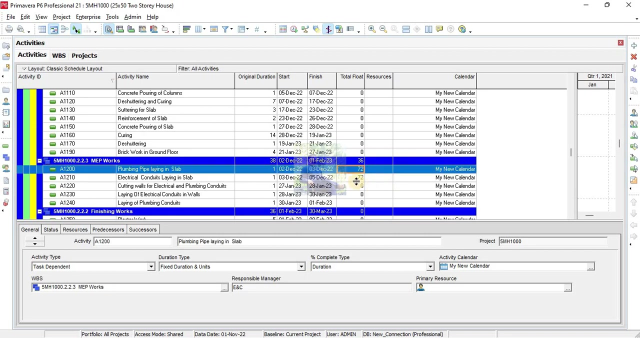 grill work. for glass work, predecessor should be tile work. for tile work and these for grill, predecessor should be this and for paint work, predecessor should be this one. now i will schedule my project from first november, so this one is 72 days float. this is uneven float. we will have to do something for this one, for this. 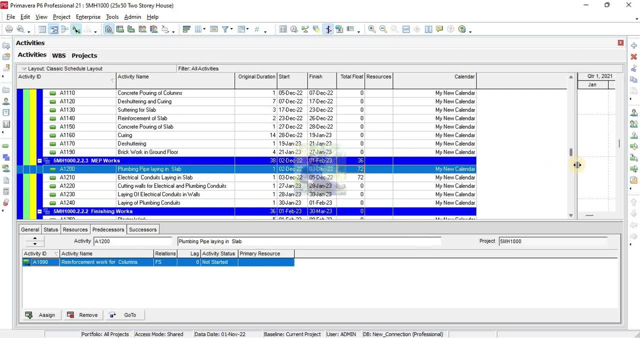 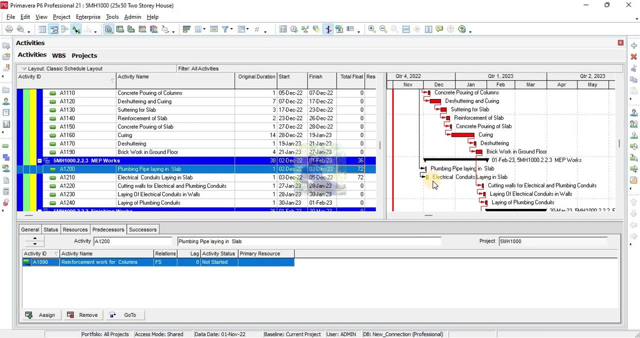 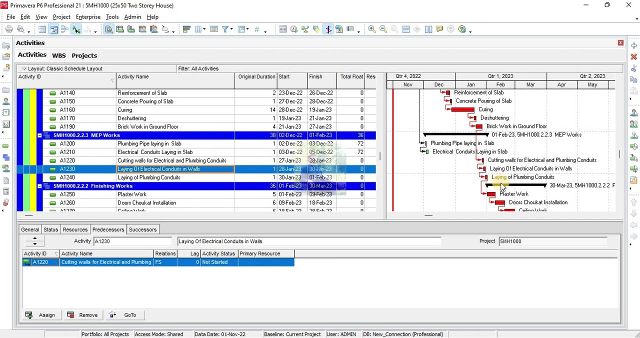 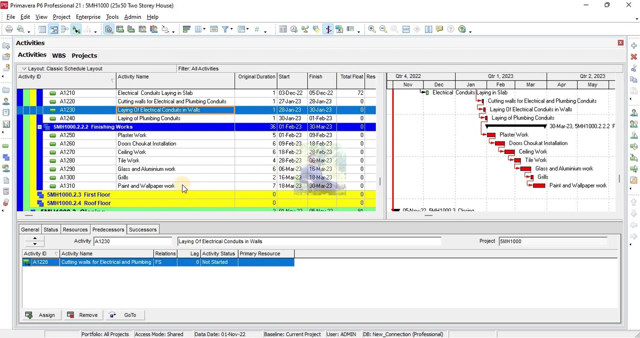 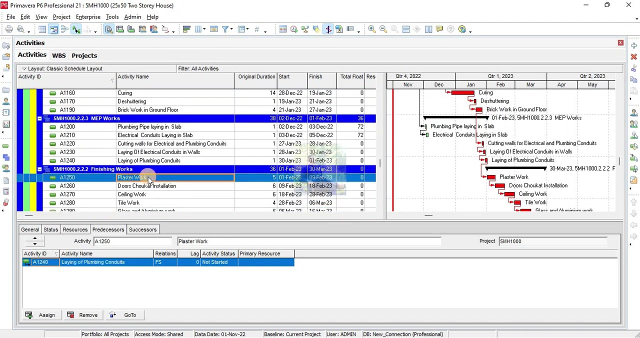 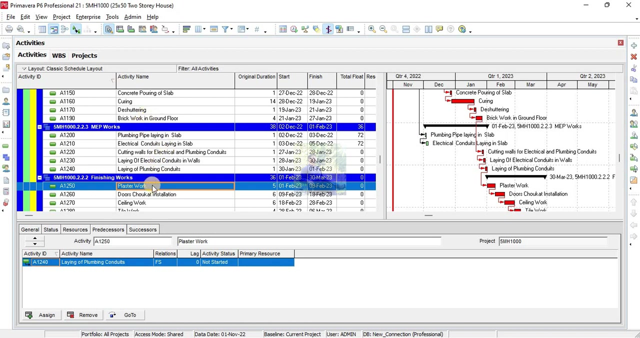 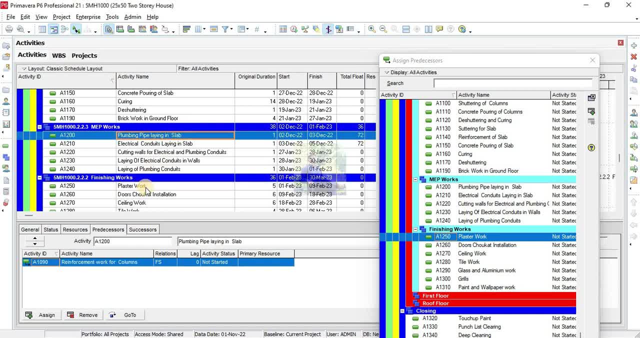 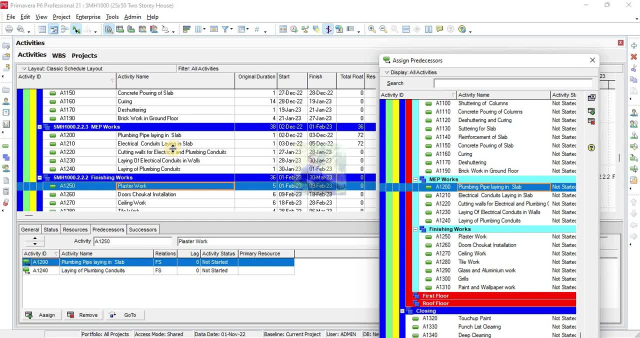 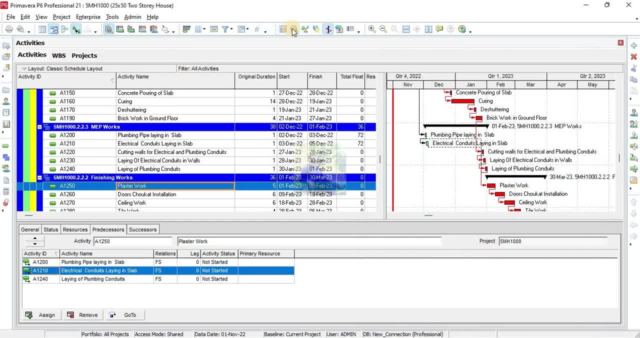 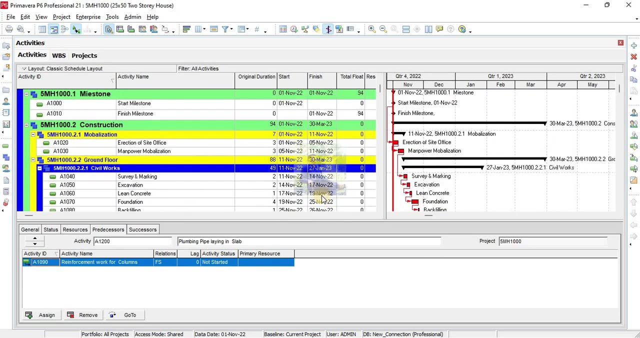 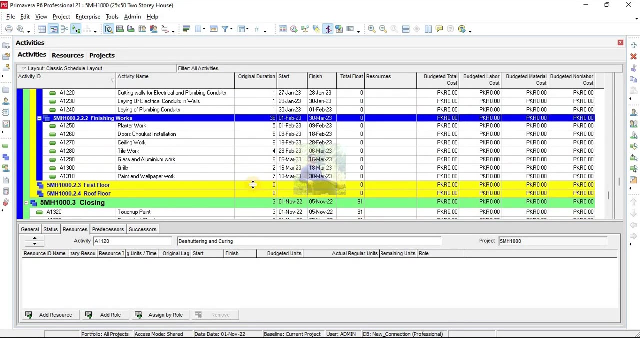 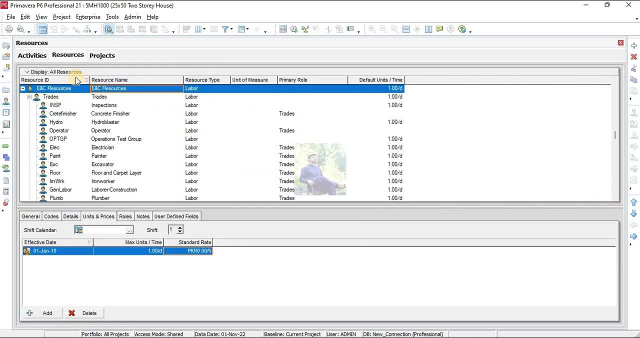 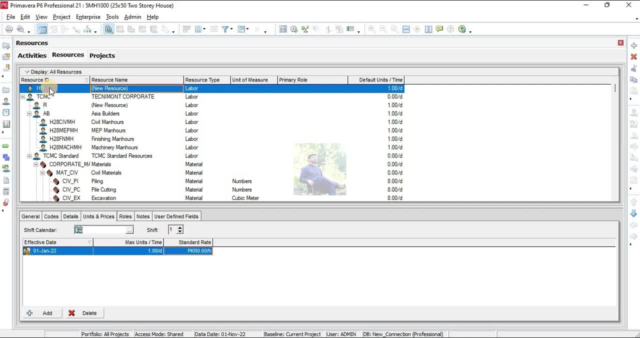 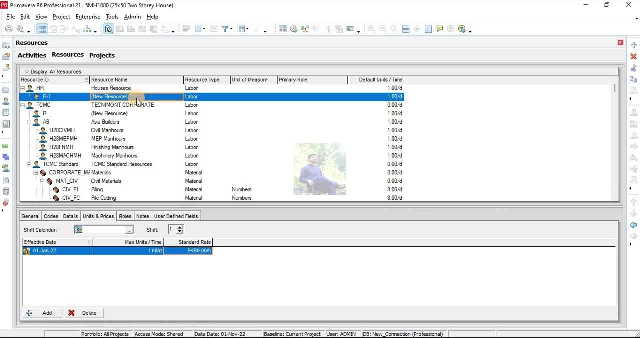 activity of these two. i want to make plaster two types of resources: civil man-hours and MEP man-hours, and this I want to make it a real resource material, and this one I want to make it machinery. so these will work 8 hours per day and standard rate, let's say, it is 50 pkr per hour, and for this 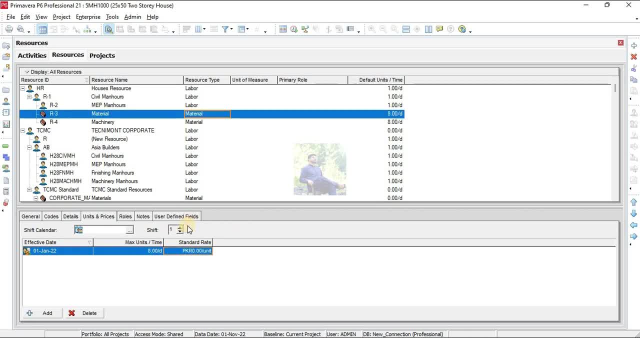 let's say 50 pkr and material it is a hundred and for a machinery it is 150. this is just simple resource pool to make our project very, very simple, but in real-time projector. this is not the scene you have to define for a material you have to. 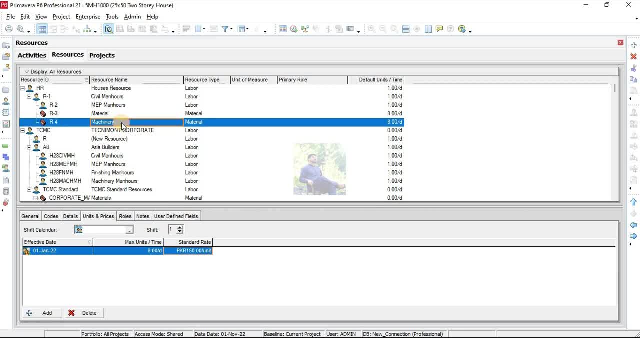 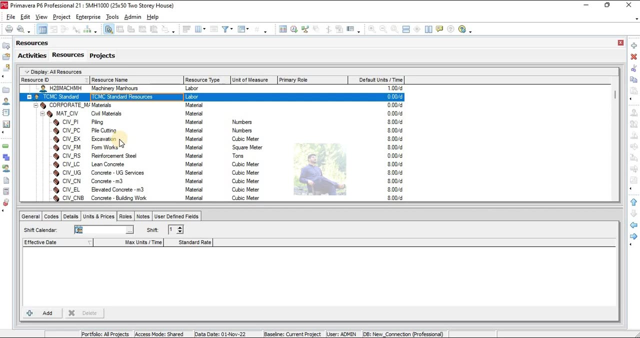 define many material resources and for machinery you have to define many machinery resources and same for man hours like this is my previous project. this was a mega project, million dollar project. duration was three hours. so for material I have defined all these: piling, pile, cutting, excavation, form works and unit of 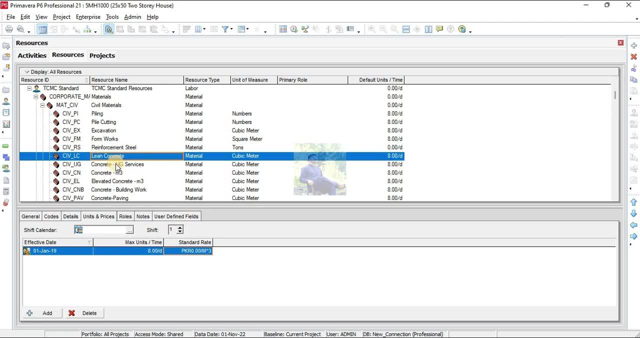 measure you have to define: reinforcement, lean concrete, concrete, underground services, elevated concrete, concrete building, concrete paving, backfilling, fireproofing, paving tiles, piping material, UG piping, field direction, and so on. you have to. these are all commodity curves and this you will need in your daily and weekly reporting. 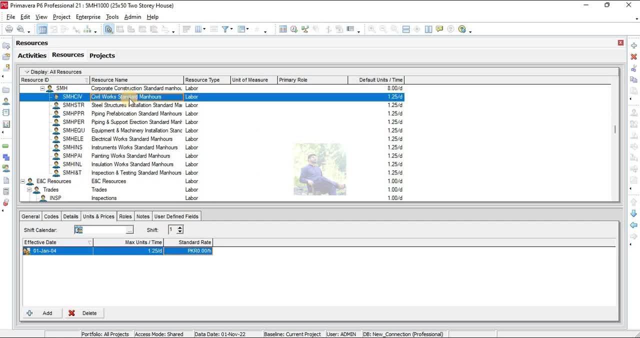 and same for man-hour. almost there were six to seven thousand working on site which are direct man-hours, so you cannot assign a man-hour. so you cannot assign a man-hour. so you cannot assign a man-hour. each by name. to simplify it, I have assigned it: civil works, standard man-hour. 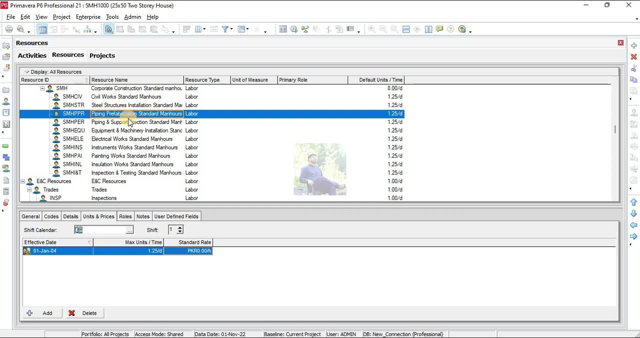 steel structure installation standard man-hour. piping fabrication standard man-hours. equipment and machinery installation standard man-hours. electrical works standard man-hours. instrumentation works standard man-hours. so from here in weekly report you will get resources to go on. so these are very important and little complex in scheduling. now we will come. 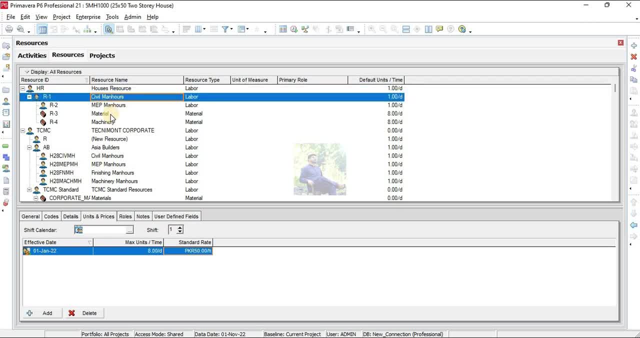 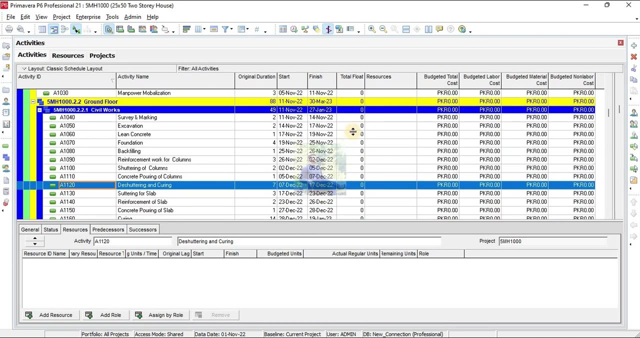 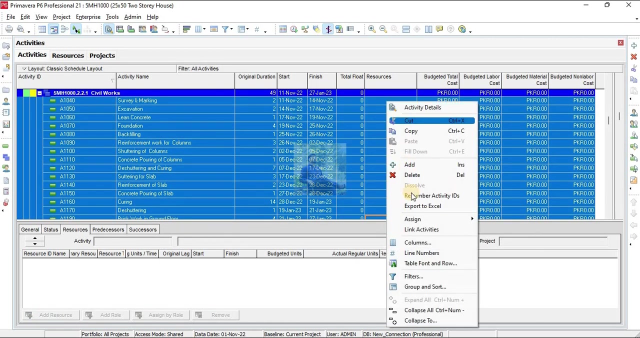 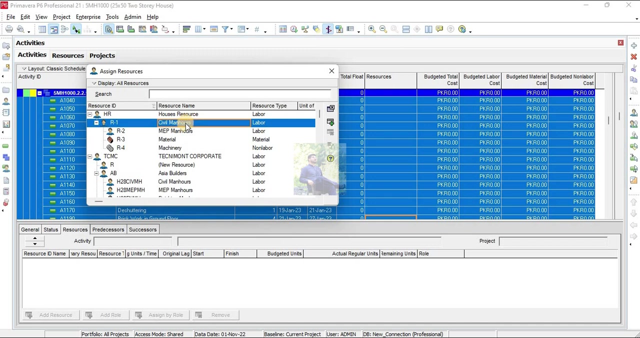 to our resource, for which is very simple: just having four resources to labor resources, and this one is machinery, which is non labor resource. now what we will do, come to our project. all these are civil activities, so how will assign resourcesığ? I will designuğa. 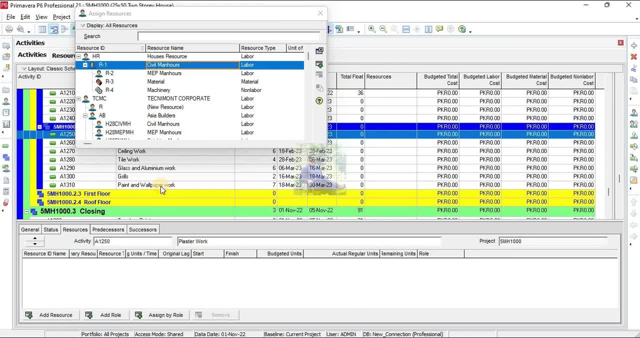 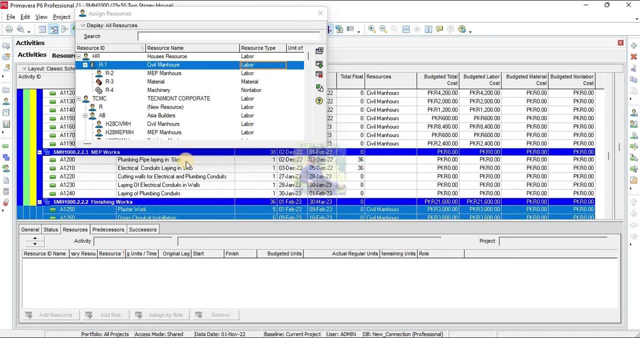 and I have assigned, and these are civil activities, civil man hours I have assigned and these hours are MEP activities. so I will assign MEP activities and these are MEP activities, have a contract numbers and these are so these activities. it will be phải ist you 10 Obasan employment and�� capital Hole there will not be embezzled so we will have to establish few other employees other. and these are civil activities. there we go. so the next is subject: here I am creating different activities for them to conduct practical work activities. so I have applied an MP activity and these are civil activities. in 2015th sub Ore, 했는데, grandma teacher and they have planned and I will assign a regard activities and these are MEP activities. so I will assign MEP activities and this will clarify specialist ed chirping лег for senior workers here on interest. 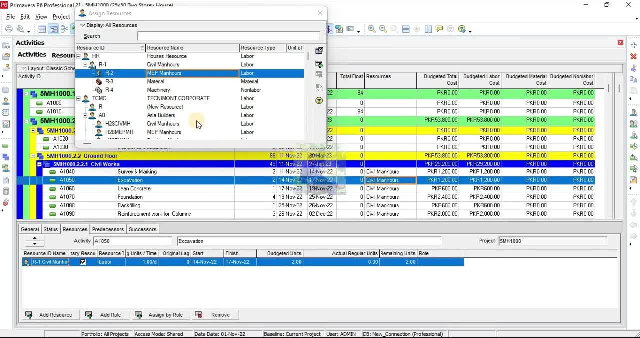 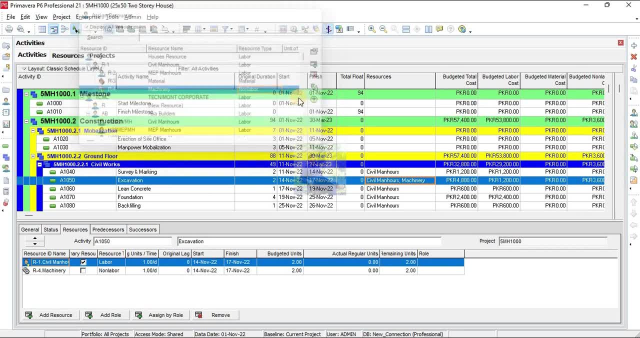 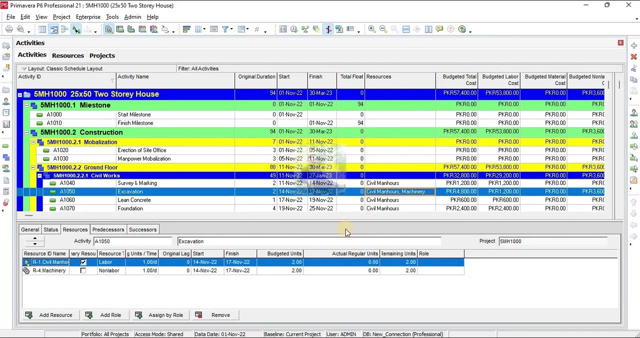 is one excavation which I will do mechanically, so I will add the machinery here. schedule it now. from here you are getting cost of the project also, budget of the project also, which is 57,400. it is because these rates are not real and I have not added material resources for. 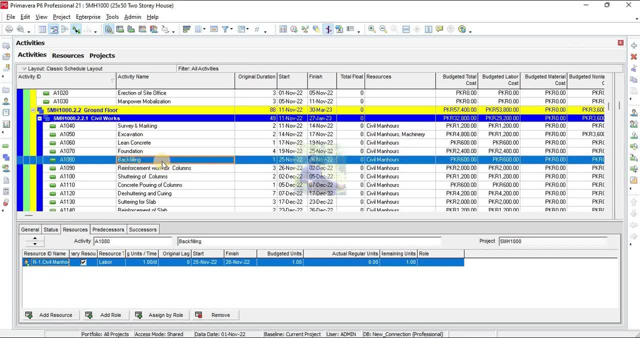 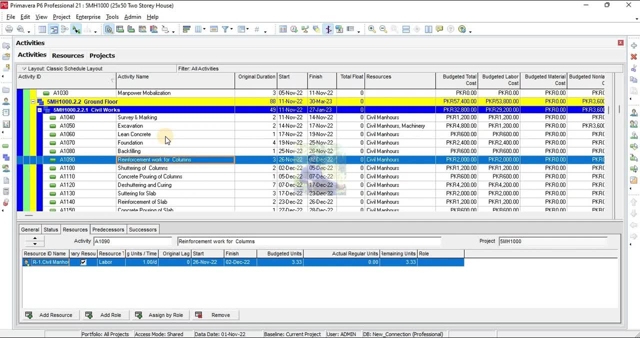 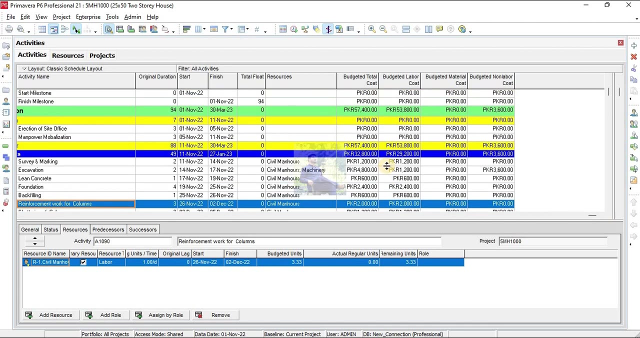 example, lean concrete foundation back feeling. there are a lot of material resources which I have not added and in next video sometime I will add all these resources to give you a complete budget of a project in Primavera and how you can do on value analysis in Primavera. so, after all these, 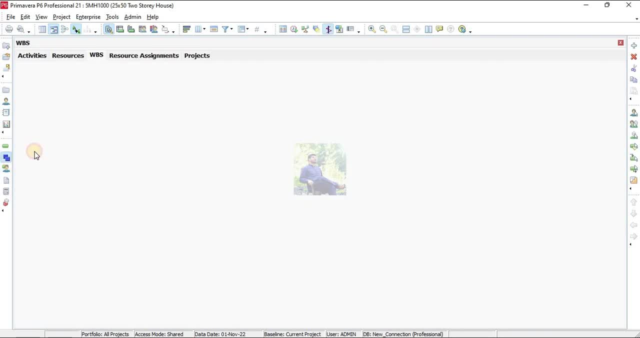 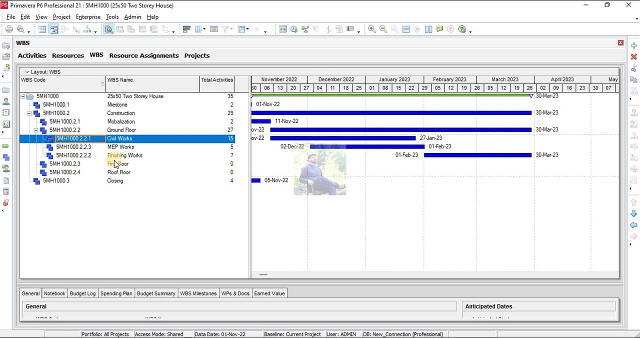 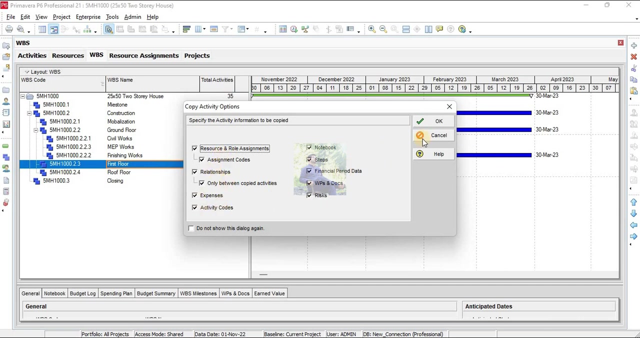 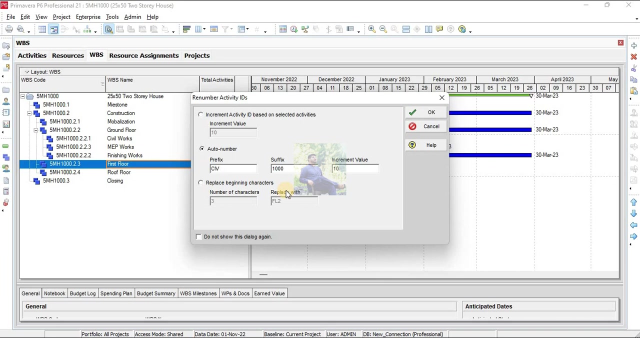 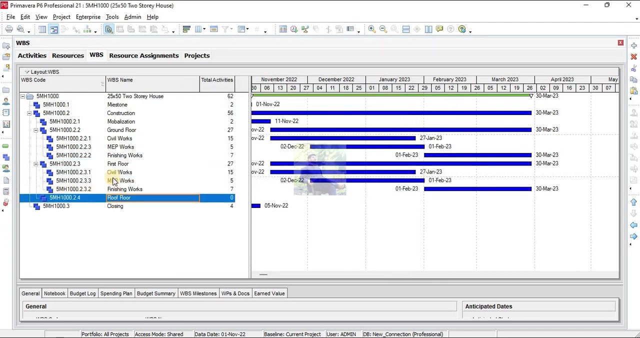 things are done. I will just simply copy these three. sorry, copy these three and paste it here. and activities also, and in activities I want all these to be copied: resources, assignments and all, blah, blah, blah, blah. these all I want to copy. and this first floor, foreign and same. copy these and paste here. 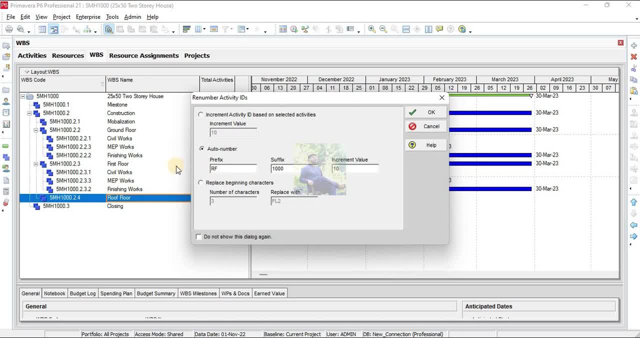 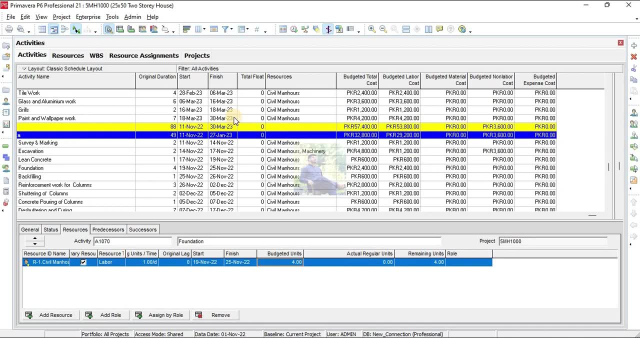 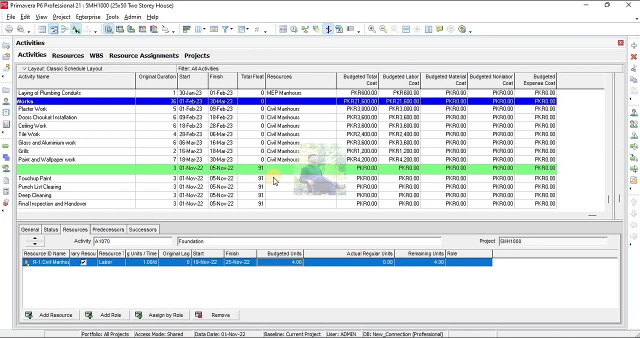 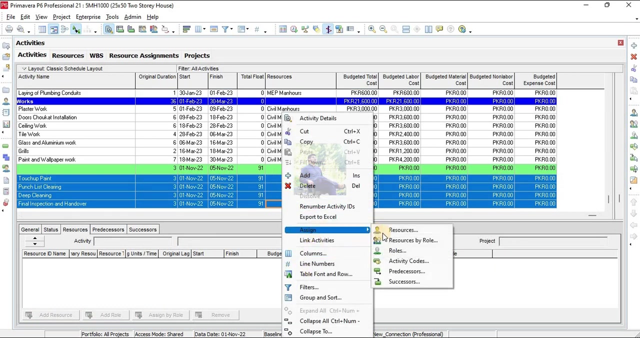 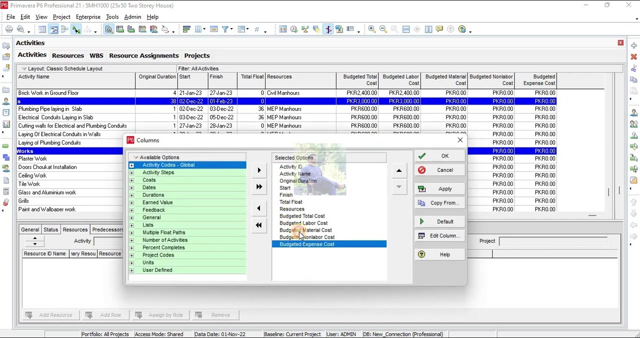 and this roof floor. so we can see here our schedule is almost completed here. I will add resources here, also assign resources, civil resources, and now I will check for open inductivities. I will hide some columns so just to make sure it's not a mistake. and it's that if I have not made changes to the agenda or I want to go back to my request. 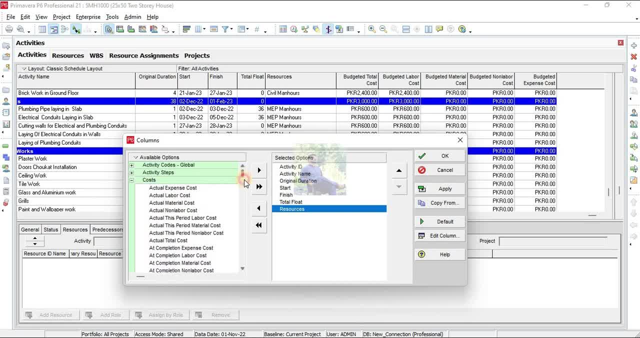 and if we start a link and then I do an update will, atleast I can open up very quickly. i don't know yet, of course, what I have been doing with this project. it's a lot harder than I thought, but I'm in a very tough time. I can't do this with the university officers, and you know. 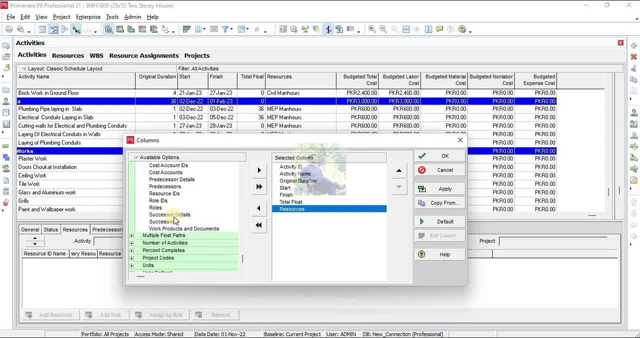 and also just that we're in such a time and space where I'm being a team and we're doing this for a very short time, so I don't think this is going to work for the rest of this call and we're going to be doing this for the rest of the day without this. so if you 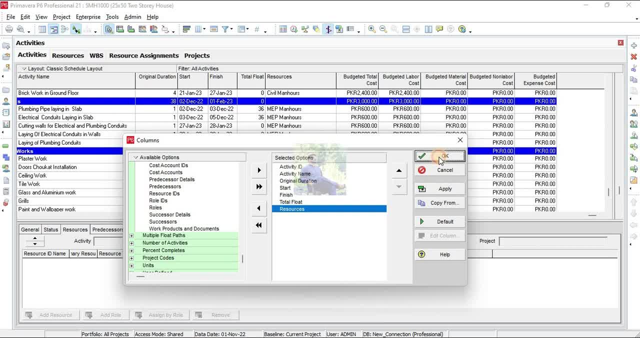 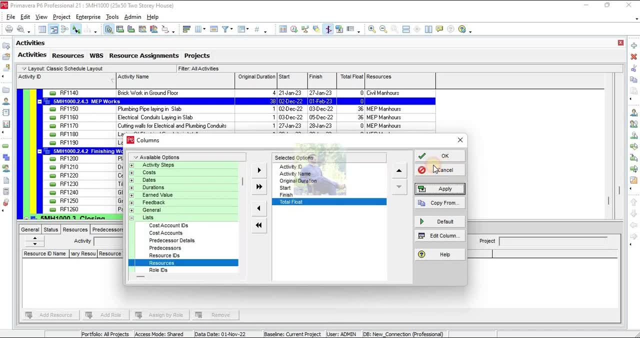 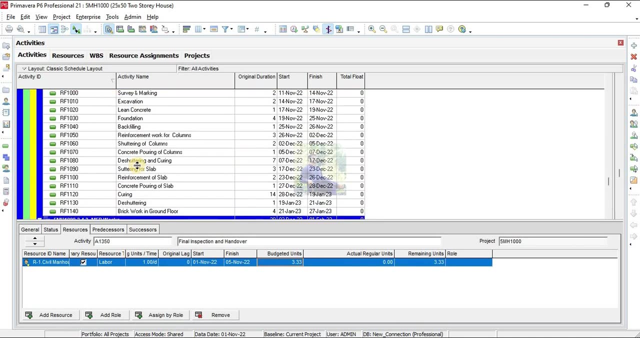 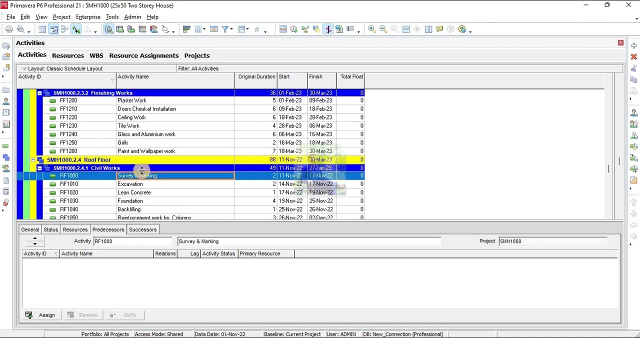 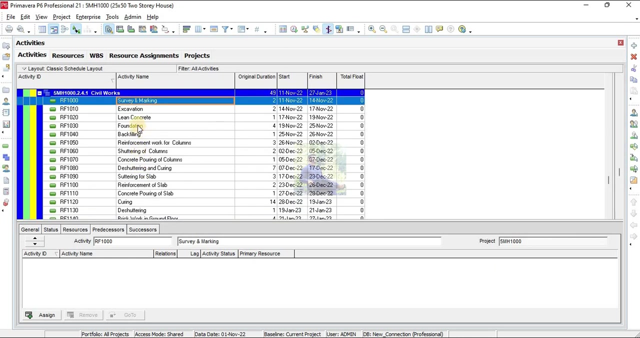 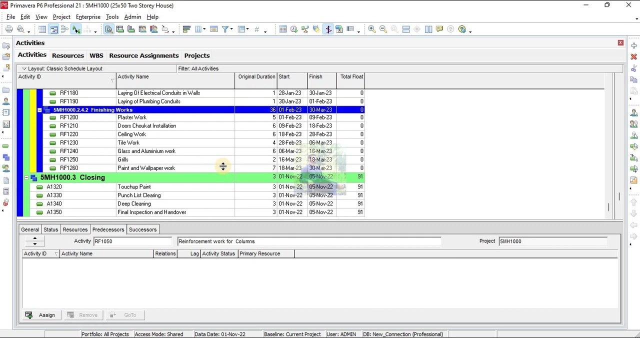 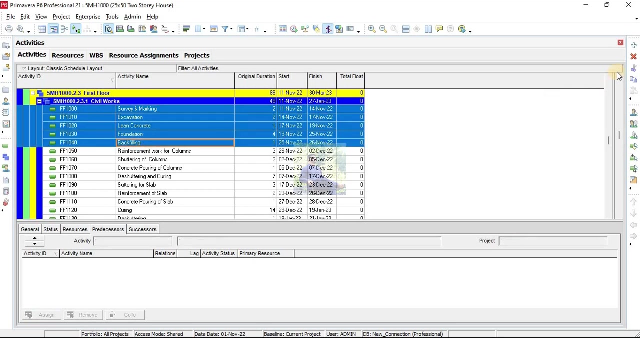 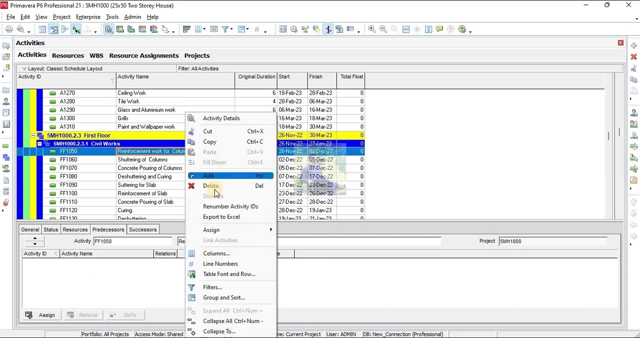 take a look at the next slide. I'm going to go ahead and and just do that window over here. and resources also. I don't want to see these three activities I don't need and similarly have these three activities I don't need. so a sign produces, or. 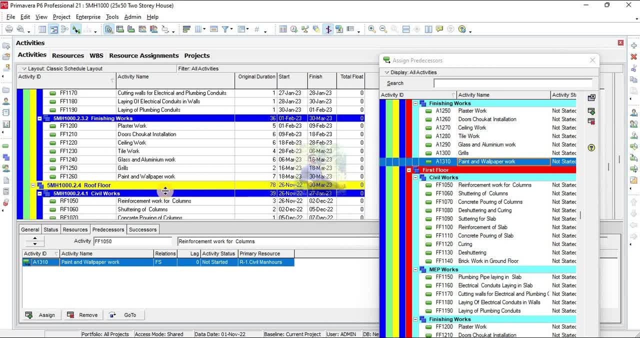 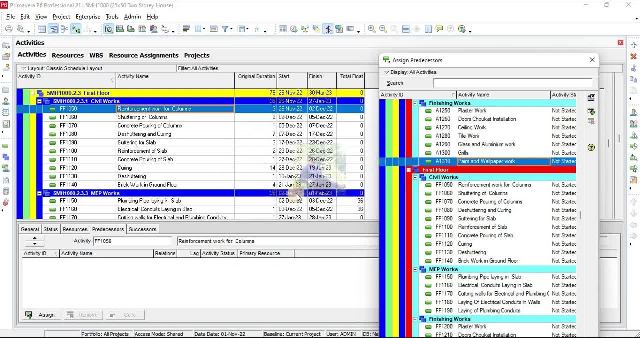 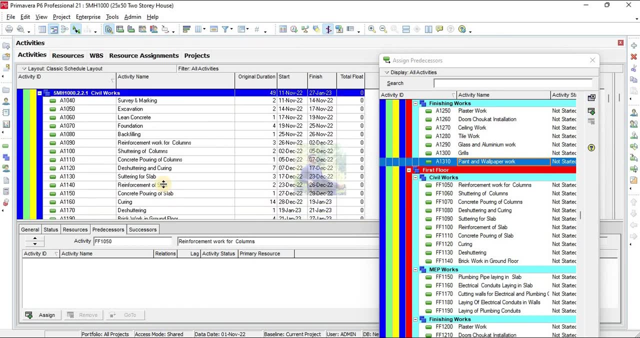 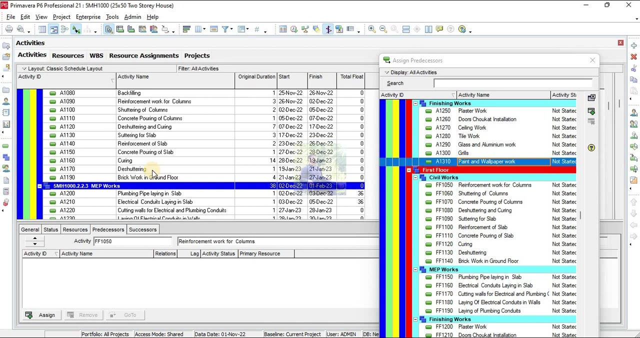 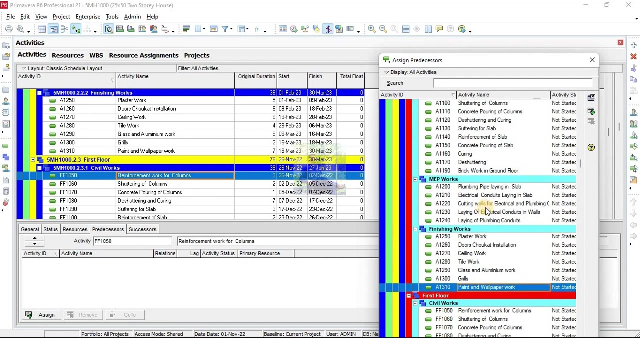 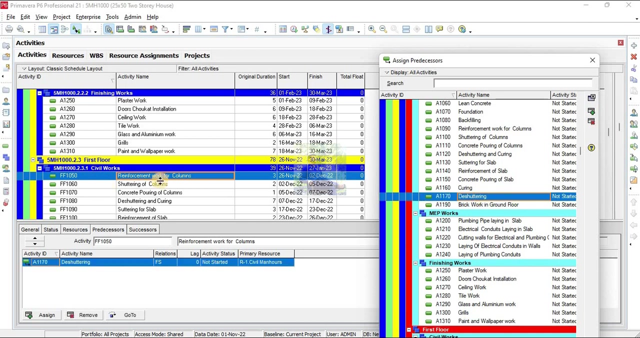 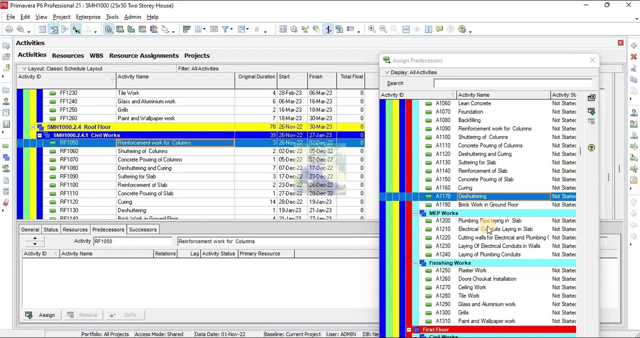 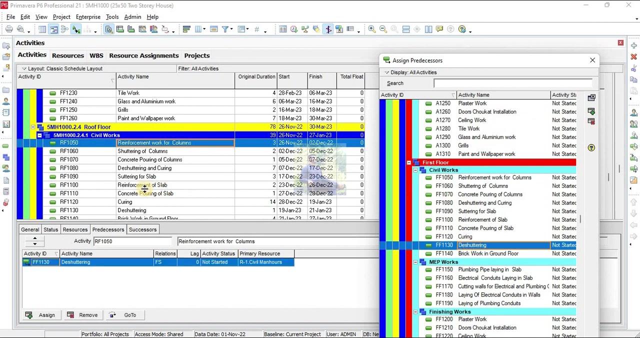 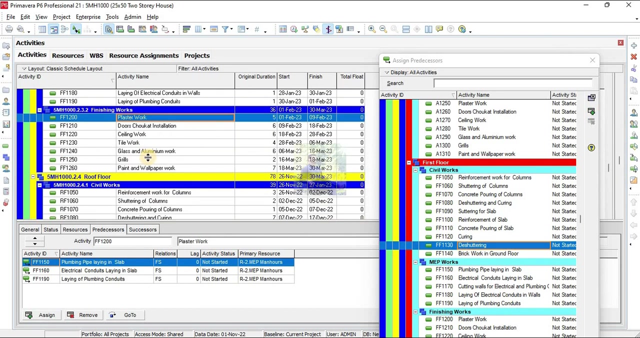 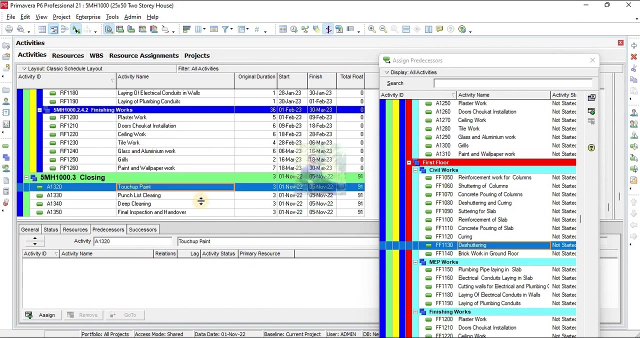 and no, in fact, after completion, after de-shortening a sign produces, or after de-shortening we can start reinforcement for columns. and same here: after de-shortening of first floor slab, we can start reinforcement, and this one of first floor slab, of first floor plan, of in this sorry. 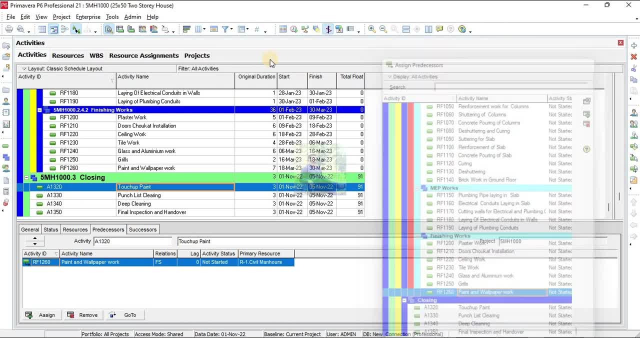 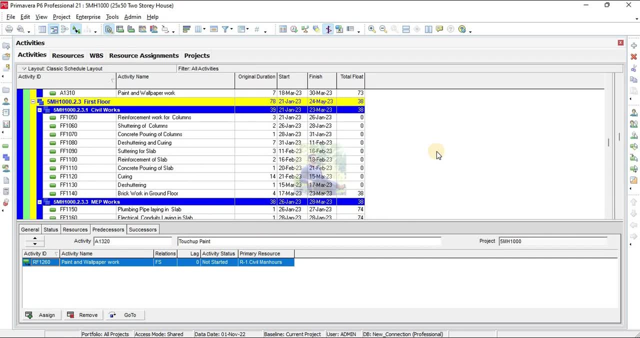 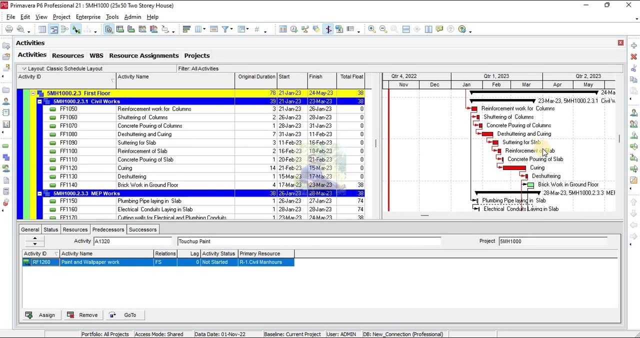 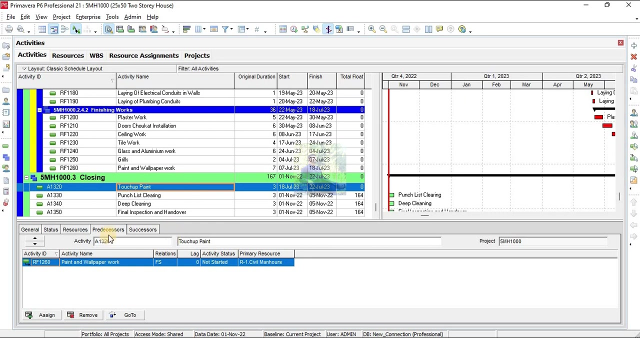 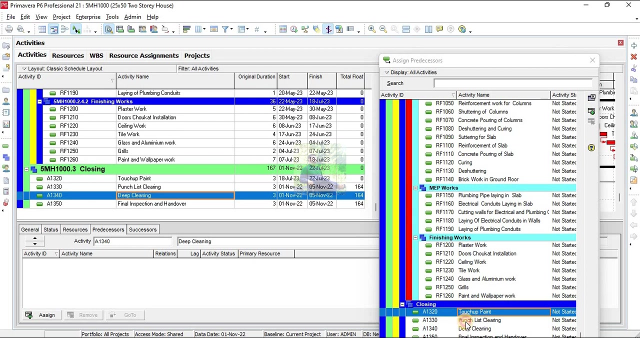 of in this: sorry, they wanna pass, they wanna pass, so they wanna pass. usually this type of ok, or this one is I in producer, or this one is I in producer. etzsoe, And for this one predecessor assign predecessor this one and for this one, this one. 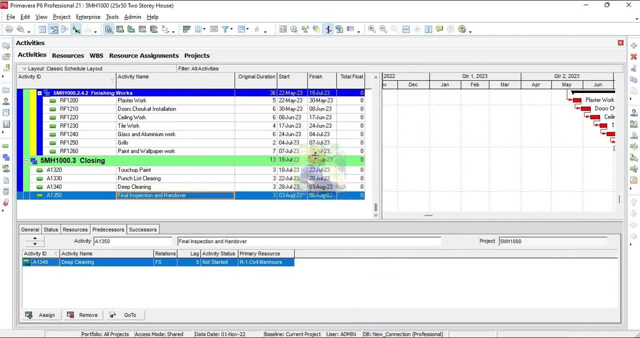 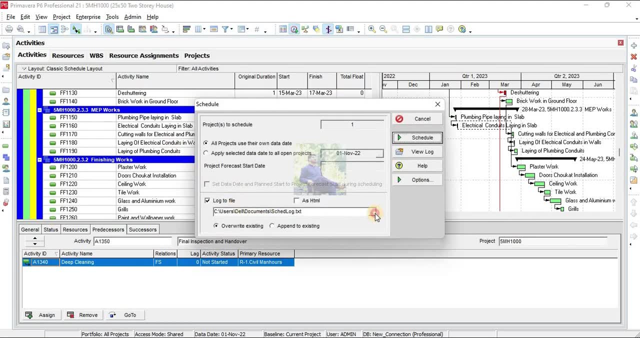 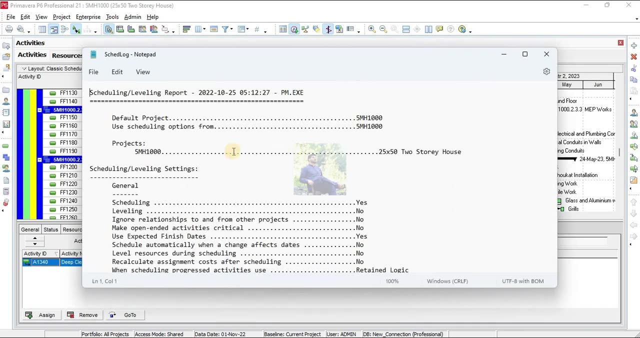 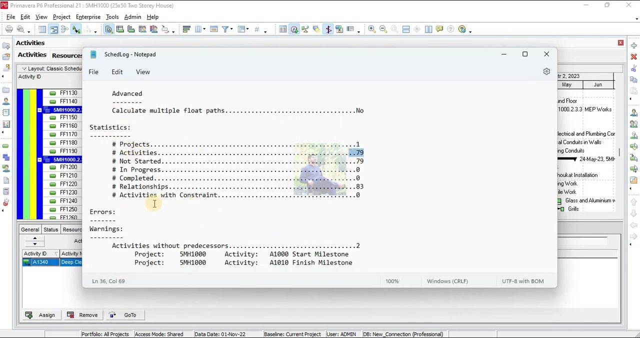 So from here we will log, from here you can get idea of your project Schedule Leveling Report, this schedule, this Productive Report. Productive Report- Productive Report Activities. there are total of 79 activities. 3 relationships in progress. there is no activity in progress. 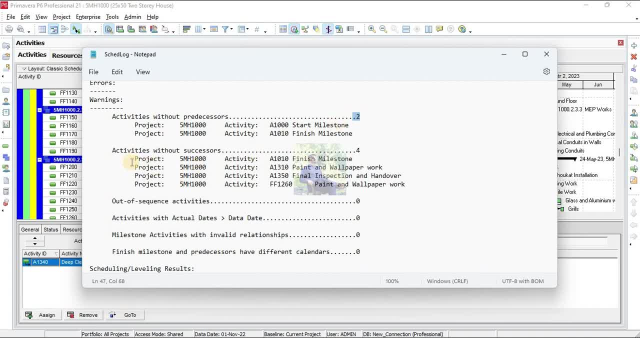 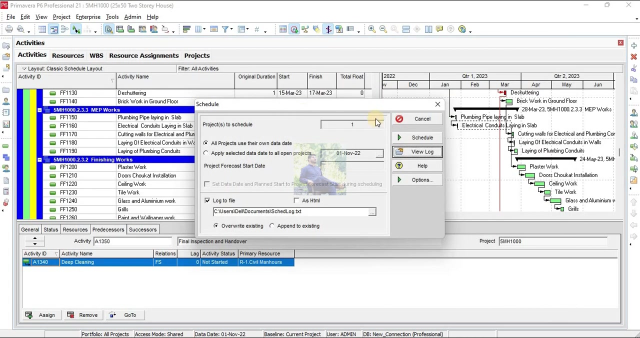 Activities without predecessor: there are 2 activities without predecessor, And activities without successor: there are 2 activities without successor. Activities without predecessor: there are 2 activities without predecessor. Activities without predecessor: there are 2 activities without predecessor. Activities without predecessor: there are 2 activities without predecessor. 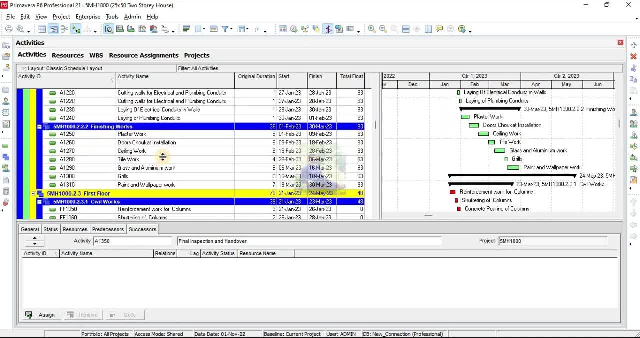 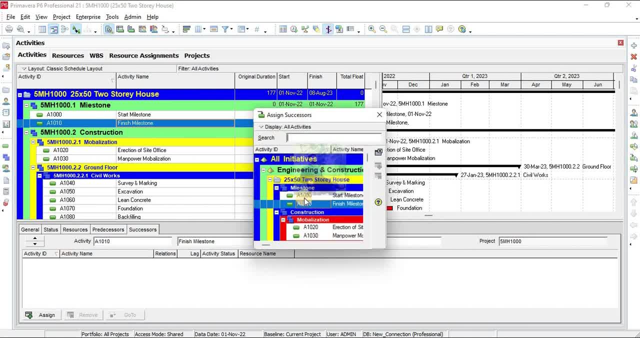 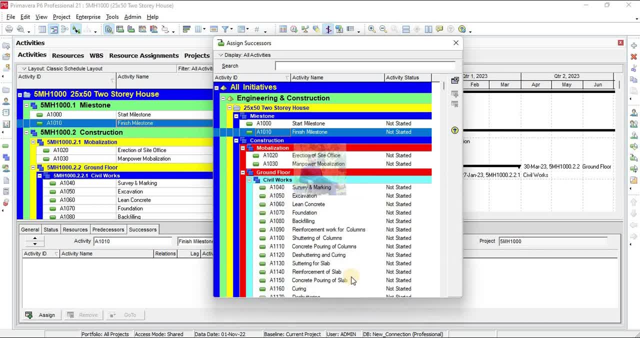 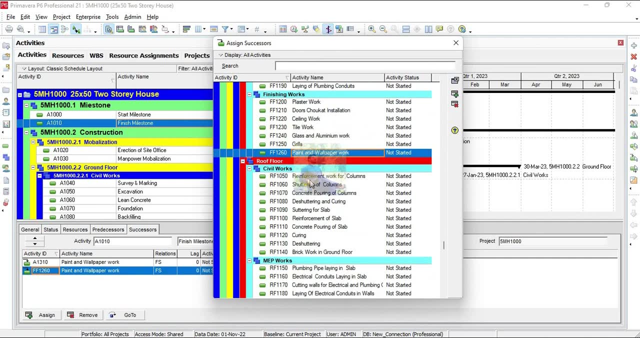 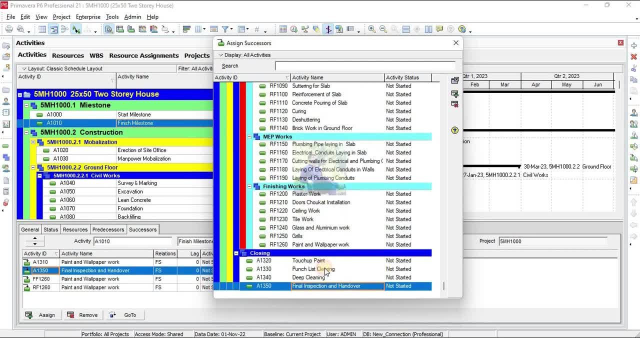 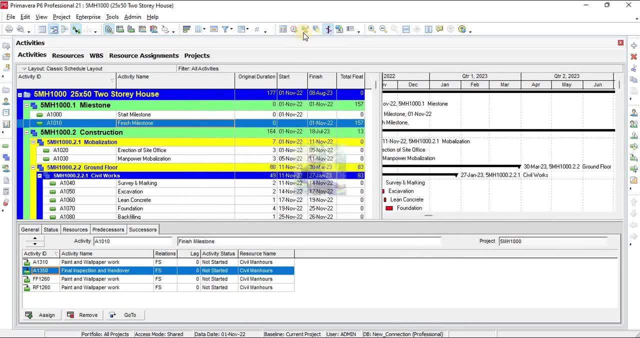 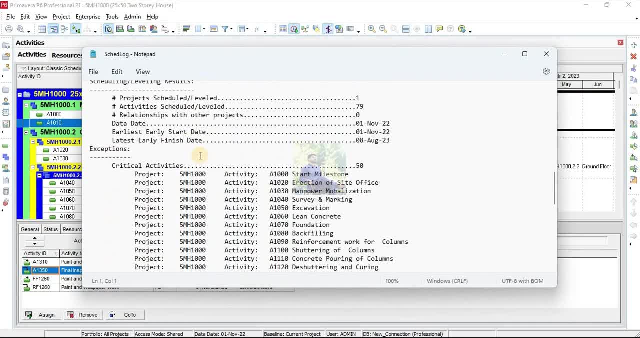 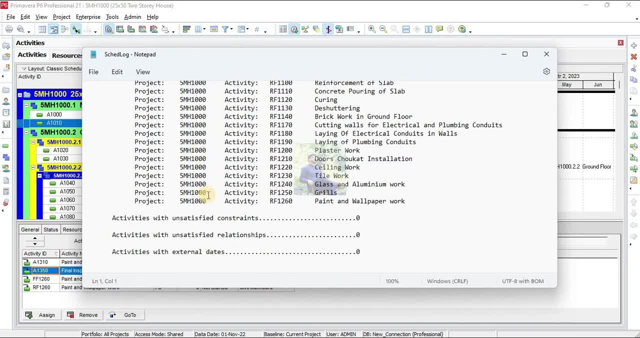 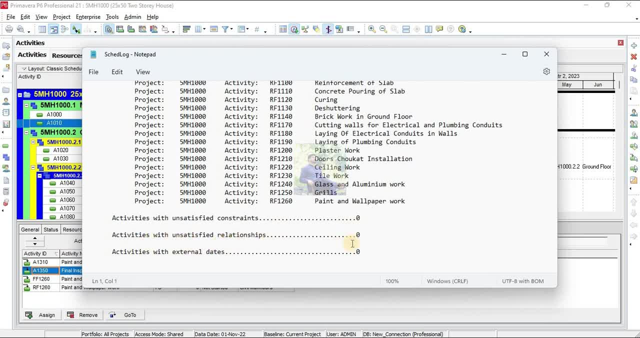 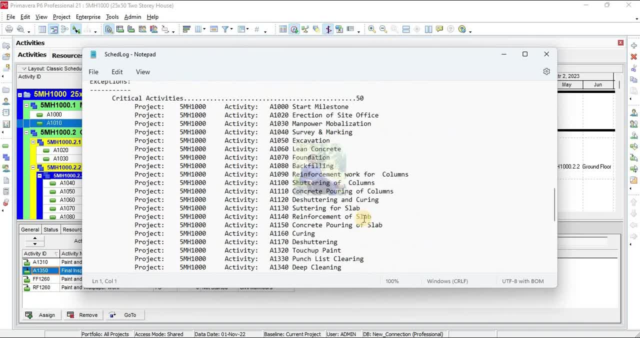 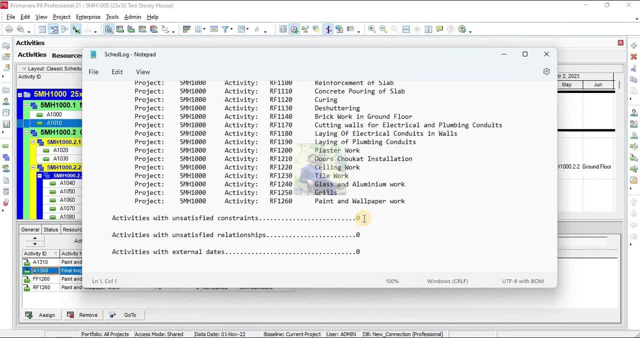 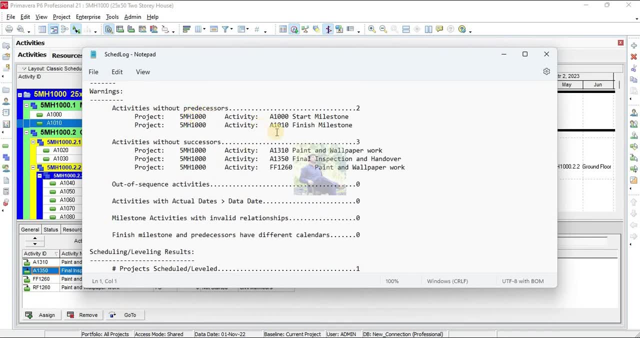 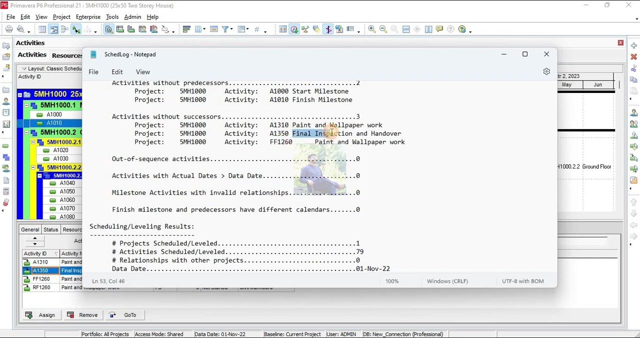 See how many open ended activities there should be. 2 open ended activities: start milestone and finish milestone. Activities without predecessor: start milestone and finish milestone. Activities without successor: final inspection: OK, they should not have any necessary objet: not England successor and and wallpaper: okay, and 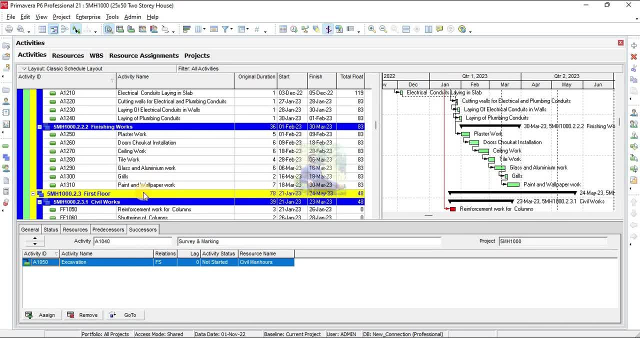 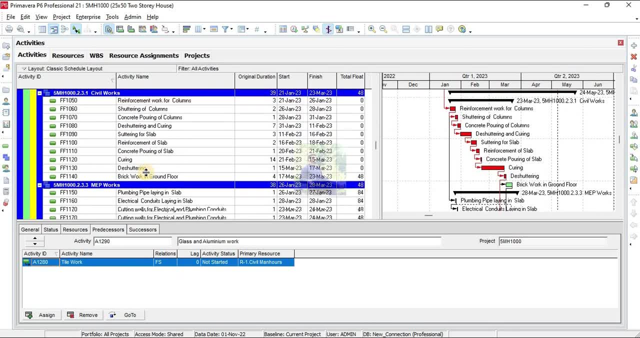 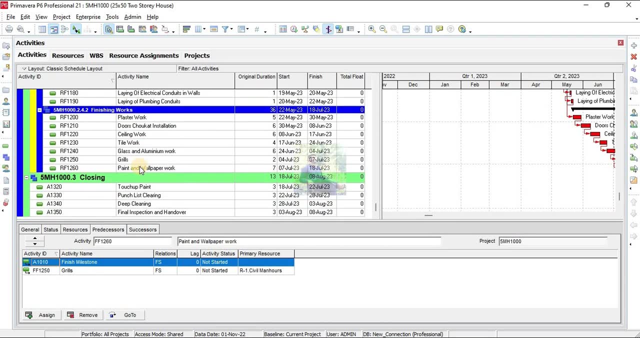 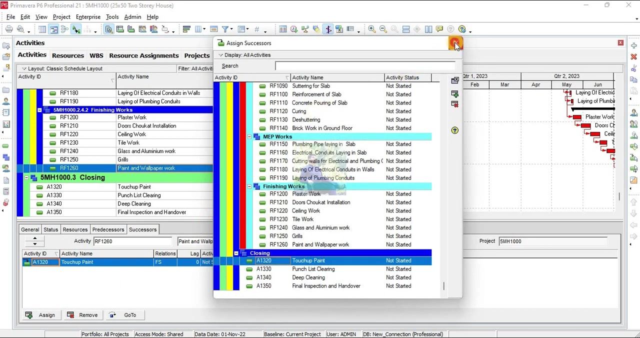 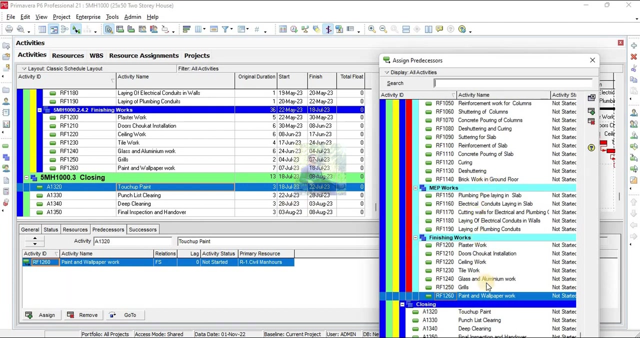 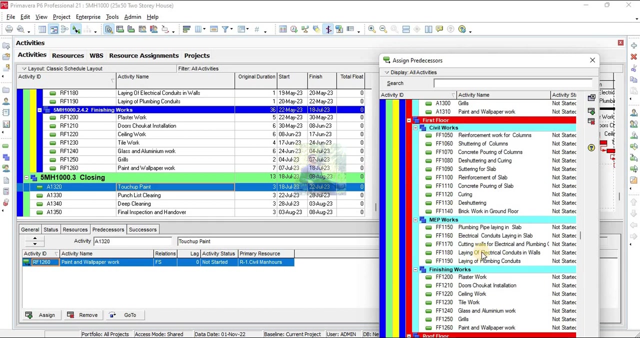 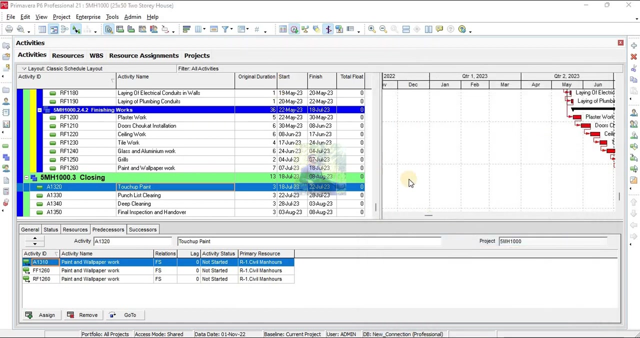 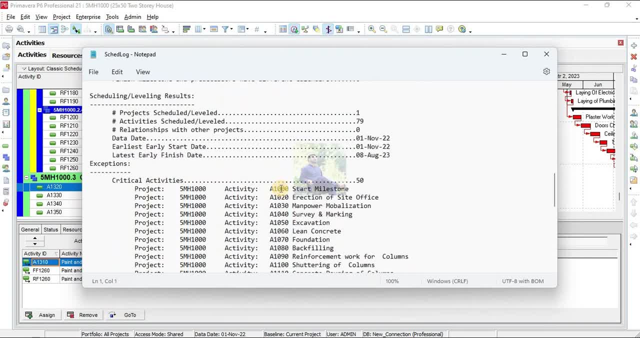 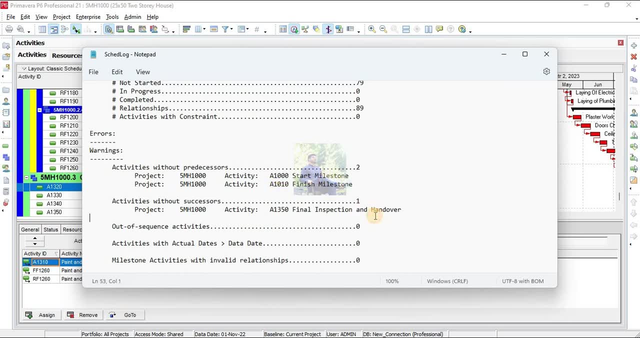 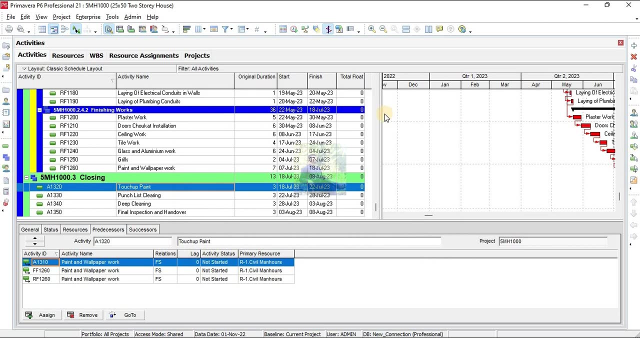 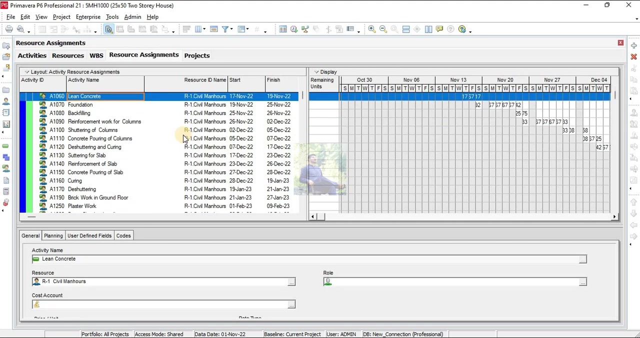 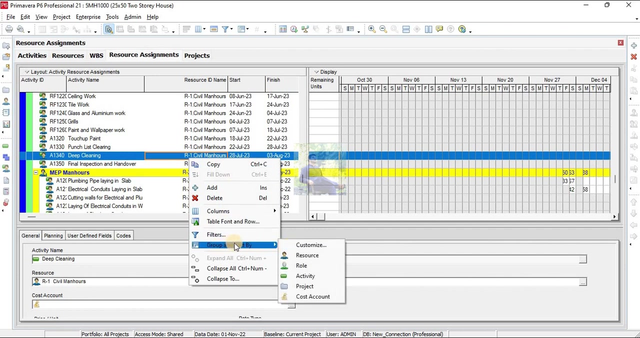 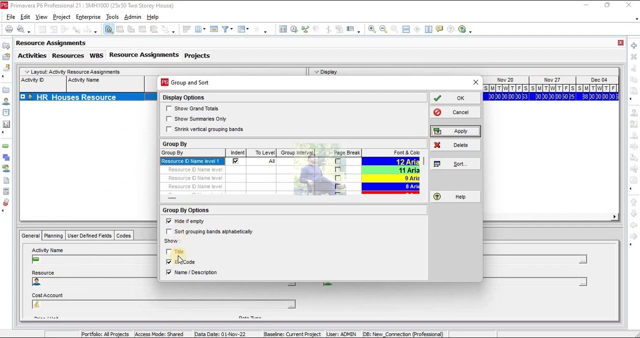 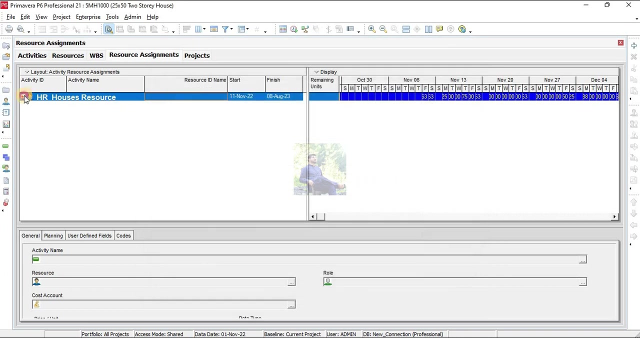 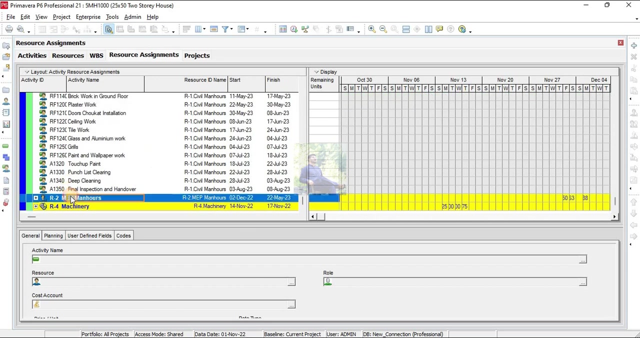 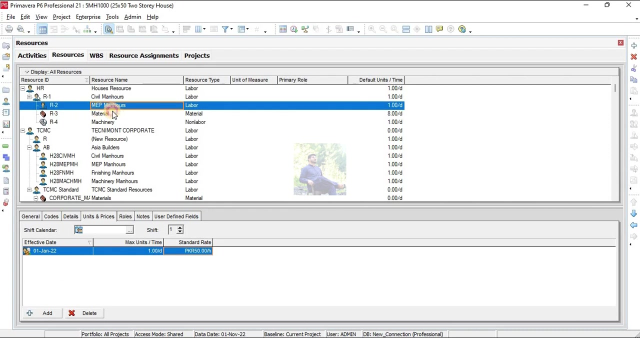 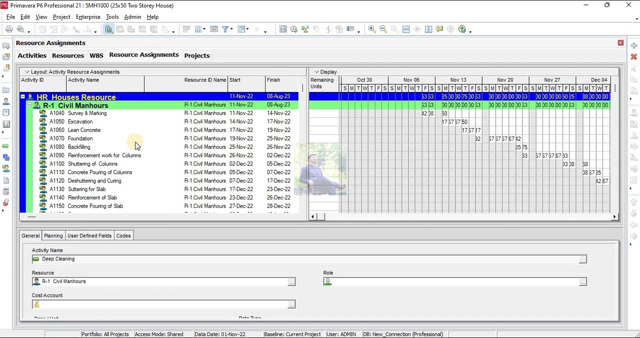 do touch-up and so now we log file activities without predecessor and activities without successor. there is only final activities without successor. so schedule seems okay now and now what you have to do: go to this resource, or okay, so make these in level. now go to resource form.